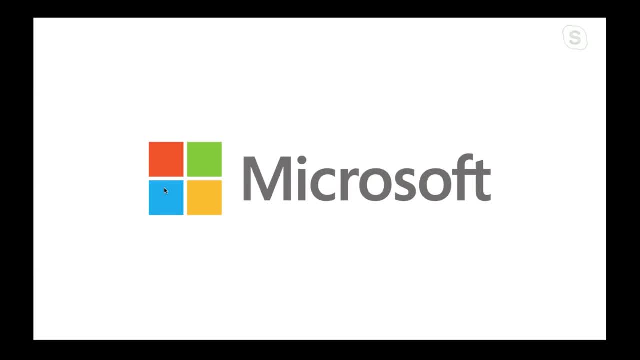 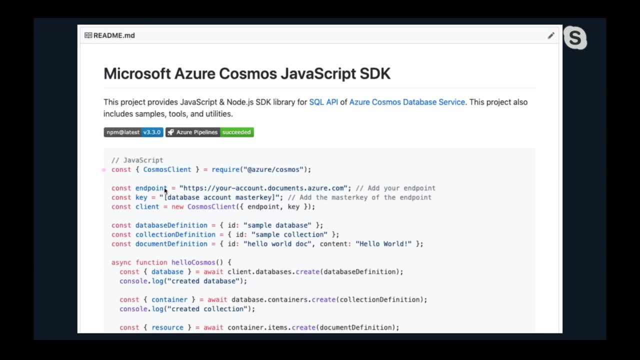 I do work at Microsoft, So I specifically work on Cosmos DB, where I maintain the JavaScript SDK. So don't worry, This is not JavaScript specific. I'm not going to be doing any complex JavaScript stuff. This is very applicable to all users of Cosmos DB for all the SDKs. 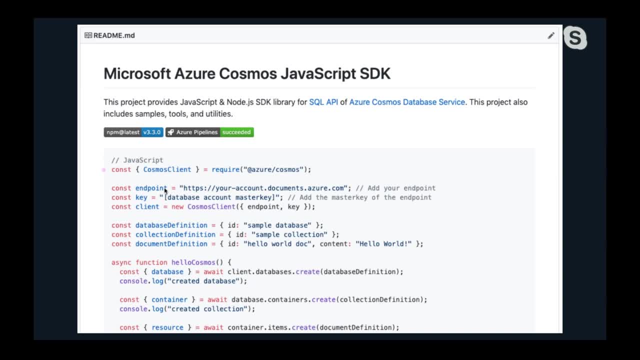 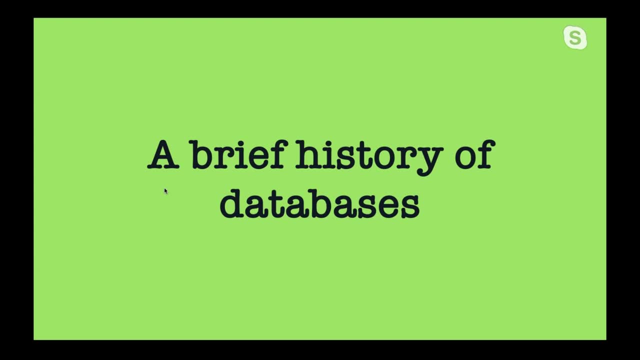 If there's any JavaScript users out there, welcome, shout out. And again, I'm talking about modeling relational data with Cosmos DB. So in order to do that, I kind of got to go back in time a little bit. I got to start at the beginning of time, talk about the history of databases and kind of how we got here. 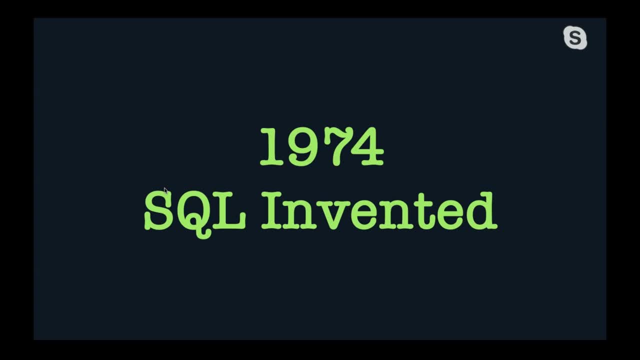 Best I can tell Googling around on the Internet, the SQL database was really invented in around 1974. So it was invented with sort of the technology that was available at that time. Let's skip ahead a little bit If anybody wants to guess in the comments the price per gigabyte in 1981, you know, relative to the same time period, it was $700,000. 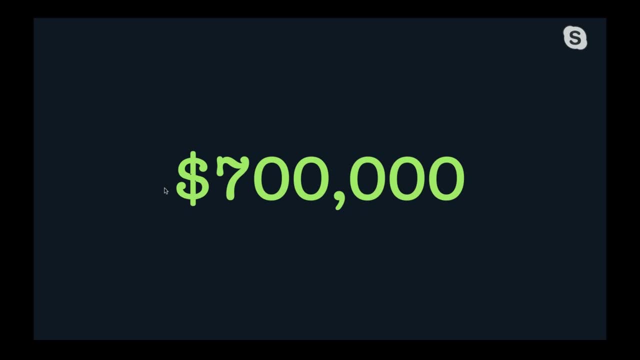 So I think this is the Apple II. So this is what it cost to store one gigabyte of data. at that time You couldn't even store a full gigabyte on one system, but this is what it would have cost you. 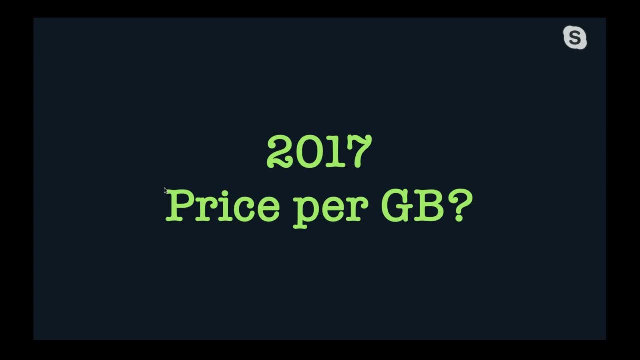 Fast forward to 2017 and the price per gigabyte two and a half cents. So clearly that's a lot. So clearly some things have changed since SQL was invented And so really a lot of these new technologies out there, like Cosmos and other NoSQL databases. they're optimizing for different things. 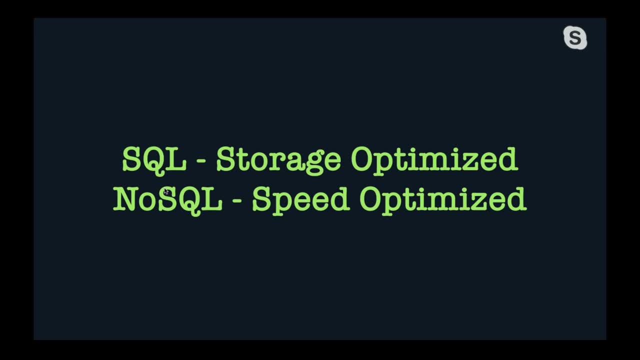 SQL was heavily optimized for storage, whereas NoSQL was optimized for speed, And that's kind of what I'm going to be talking about today is like how the way we model data is going to change for NoSQL Specifically, I'm going to talk a lot about Cosmos. 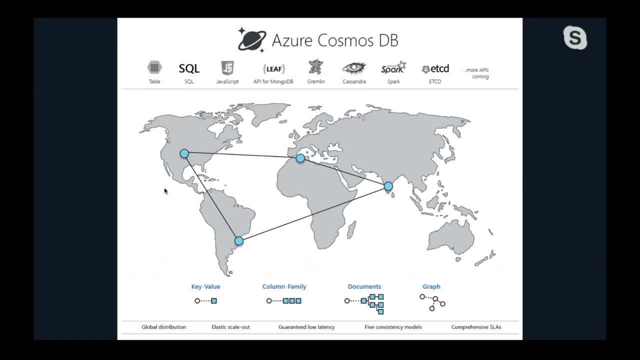 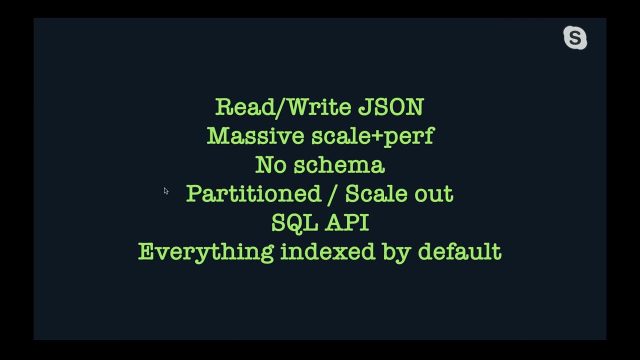 Cosmos is Azure's NoSQL database product. It's globally distributed. It's a document store. It has this fantastic ability to scale out, take your data and distribute it between different regions and copy it between different regions. Here's kind of like the important bits that I think are important as a developer. 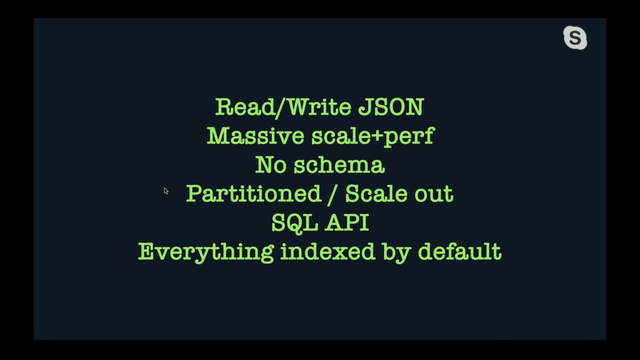 You read and write JSON. It's just a document database. It has this massive scale and performance. it's capable of No schema, so it's schemaless. compared to a SQL database, This is going to be a little bit different And it's also partitioned. 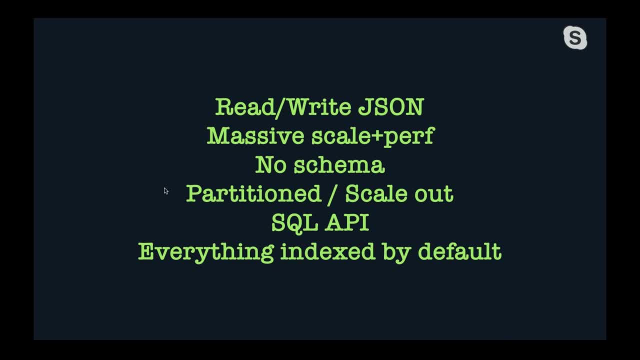 So it scales out. I'm going to get into partition in a little bit, But it has a system where your data can exist on different machines. It also has a SQL API, which is really cool, And everything is indexed by default, which is also a really neat feature and pretty unique to Cosmos. 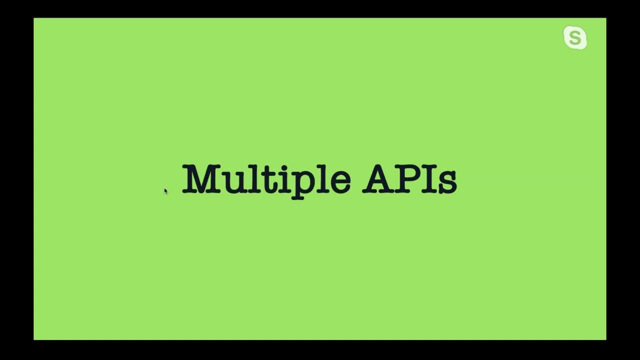 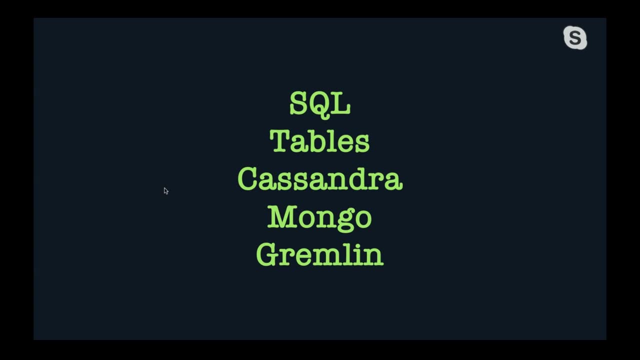 Digging in a little bit more into some of these aspects, the multiple APIs So we have- these are our main APIs at this current moment. We have SQL. It's kind of like the primary original API of Cosmos. There's a tables API. 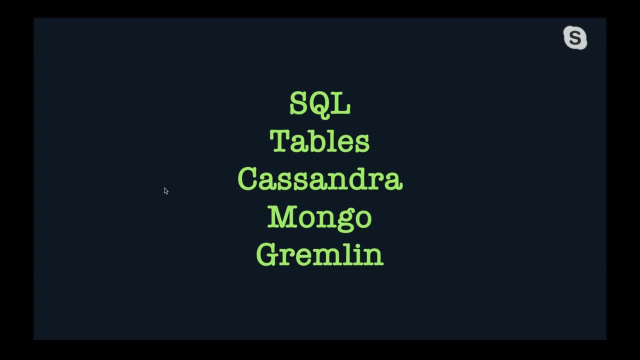 There's a Cassandra API So you can talk to Cosmos like you would any other Cassandra system. This is really great. if you're coming from an existing workload or existing application that uses Cassandra, You can just use Cosmos via all your Cassandra drivers, which is really cool. 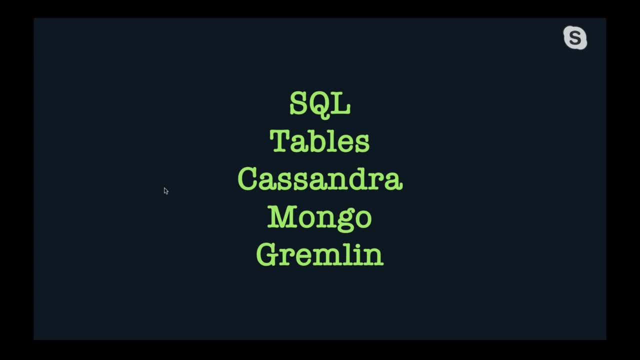 Same thing for Mongo and Gremlin. These have been built on the open source tools that are already out there, So you can use all of our driver or the open source drivers and existing database SDKs for talking with those tools. We also have some cool things in the works. 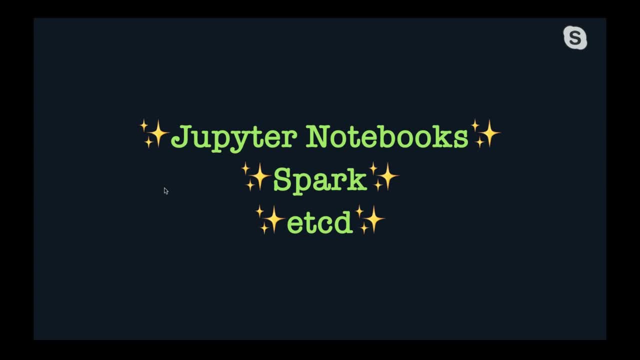 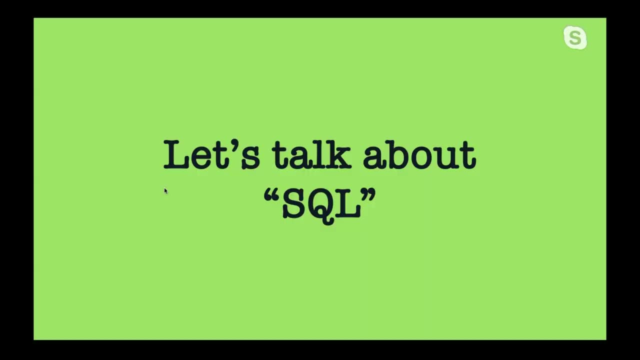 I believe this just hit public preview. Jupyter Notebooks, as well as Spark, is on the horizon and etcd as well. But today I'm really going to be focused on the SQL API. I'm going to be talking about how to do relational modeling there. 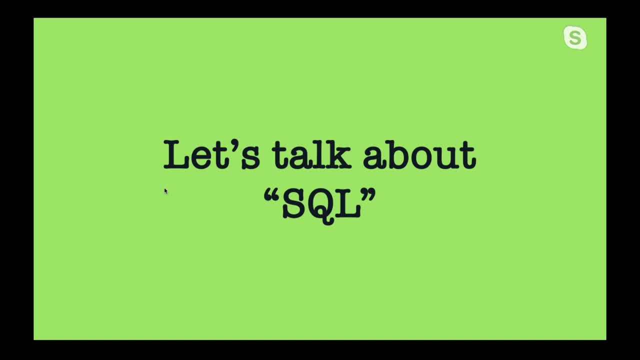 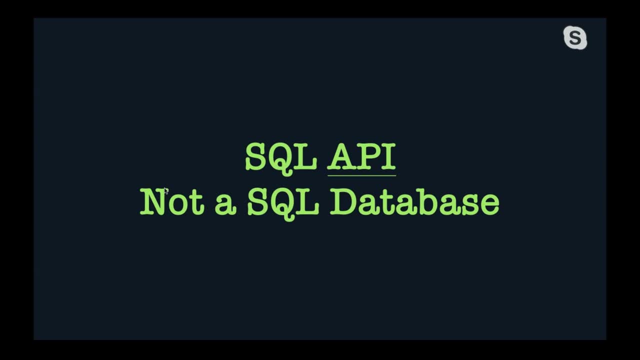 It's kind of the one that frequently gives people the most hiccups. So the first thing to understand is: it's a SQL API. It's a SQL API, but it is not a SQL database. This definitely trips people up. They come to Cosmos. 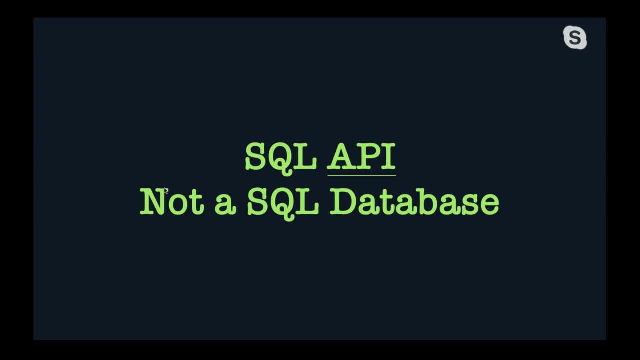 They start raising really complex SQL queries And either they don't work or they're really not very performant because under the hood it's still not a SQL database. We're just kind of exposing this SQL layer on top of your documents, So something to definitely be aware of. 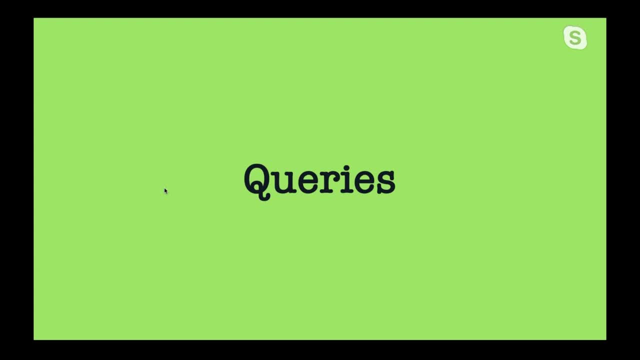 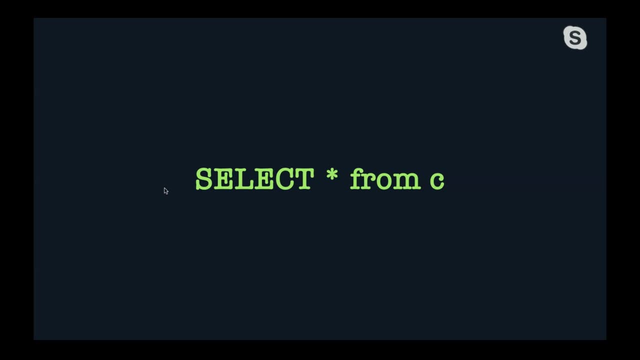 That leads us into Cosmos Queries. So Cosmos Queries, they're SQL. This is probably the most basic one you can run. These are from C. You can select individual attributes. You can also select filters based on where clauses. You could do things like picking a do at that's greater than today. 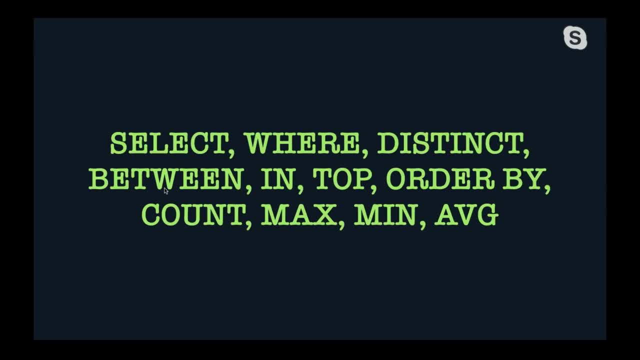 You can order by. There's a bunch of different stuff. This is not the full list of SQL that we support, but this is kind of the big ones people tend to use in practice. Select where distinct order by Count, max and min and average. 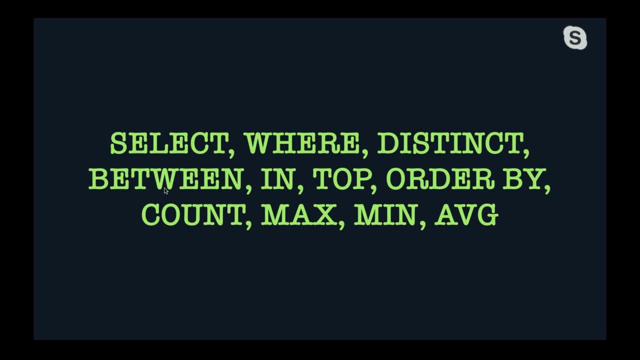 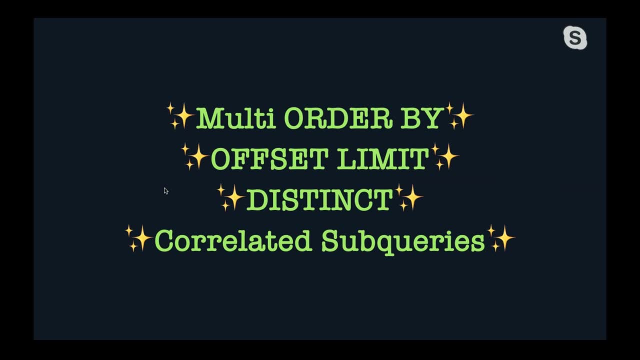 These are all aggregate queries, So there's some support for aggregate queries, which is pretty cool. We've got some other cool stuff on the Verizon. I want to mention Multi-order by is coming Offset and limit we already have out. 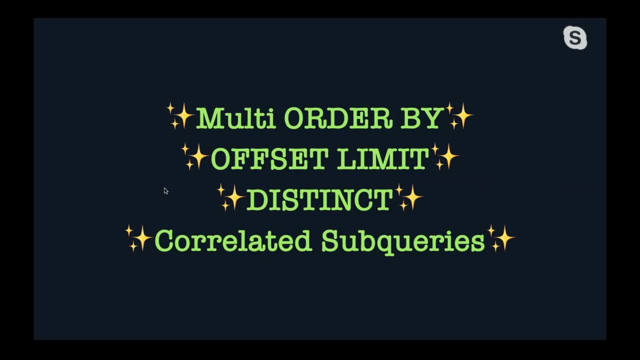 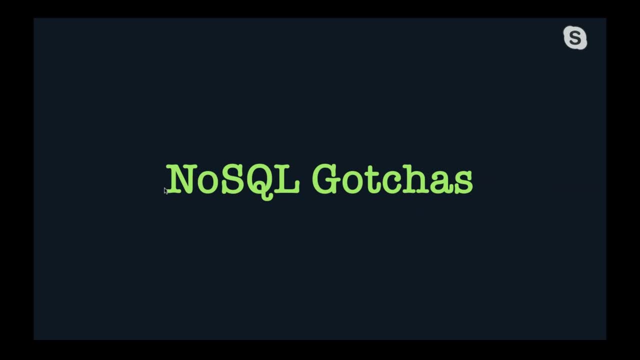 Distinct. we already have out- I mentioned that earlier- And then correlated subqueries as well. So kind of be on the lookout for those things that are relatively new to Cosmos. But because it's still a NoSQL system under the hood and it's a document database, we still have the same kind of gotchas that can happen with any NoSQL system. 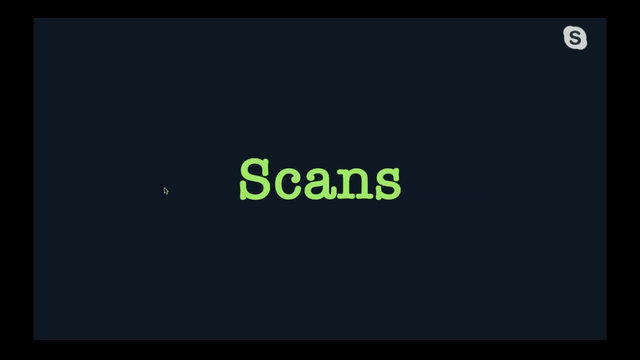 So we're going to talk about that. So let's talk about the NoSQL system, And those are two things. The first thing is scans And Cosmos. because we index everything by default, we kind of tend to avoid this problem. 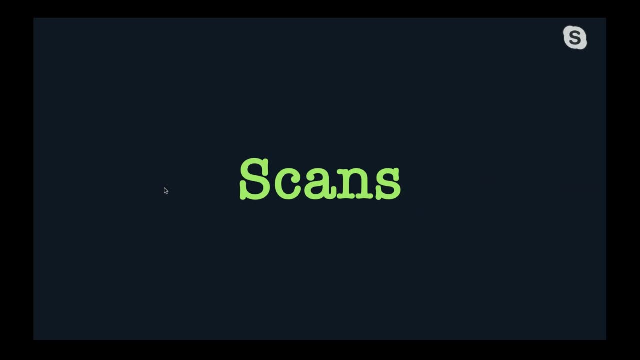 It's still possible to do a scan, but it usually doesn't happen out of the box, So other NoSQL products can worry about this. We don't really run into it too much, But the big one is cross partition queries. This is both one of the unique features of Cosmos as well as one of the Achilles heels that people will have in their application. 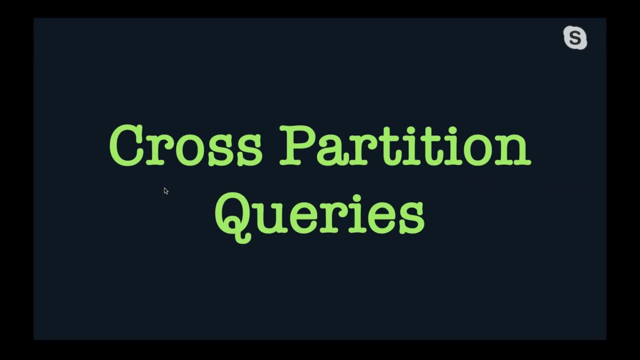 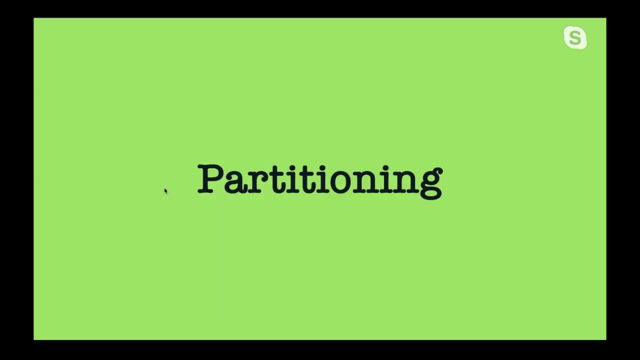 Cross partition queries. Cross partition queries is when you're talking to multiple physical machines in order to execute an individual query. Now I'm going to jump a little more into partitioning and how that actually works, so you can understand both what I mean by cross partition queries and also understand how those are executed by Cosmos. 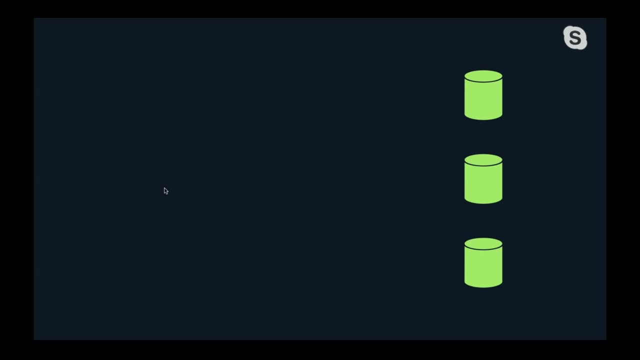 So imagine the Cosmos backend. It has machines in different regions, potentially, but even in one region, multiple machines that are storing your data, And what ends up happening is that a hash of your partition key that you provide as part of your data comes in. 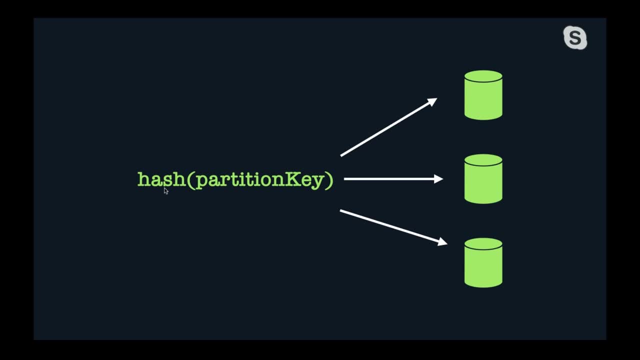 And that determines where that data lives, which machine it lives on, And then ID is the thing that uniquely identifies that document on an individual machine. This is all transparent to you. You don't have to really worry about machines. You don't have to have instances of Cosmos running. 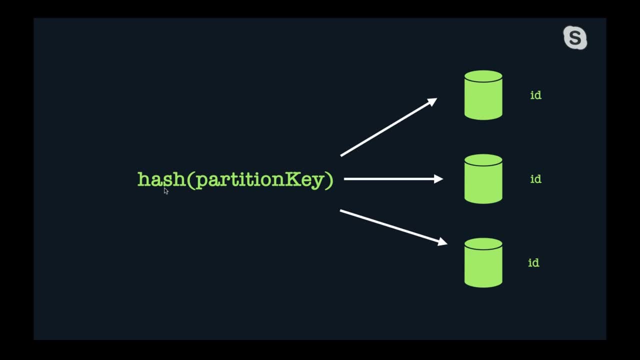 It's all serverless, But it's important to kind of understand how it's working behind the hood so we can do things in a performant way. So the important kind of takeaway here is that a document is uniquely identified by ID and partition key. 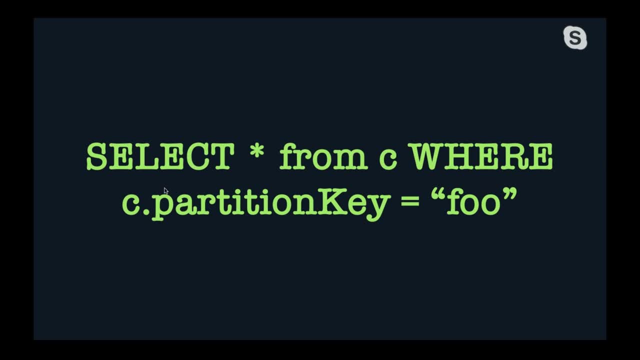 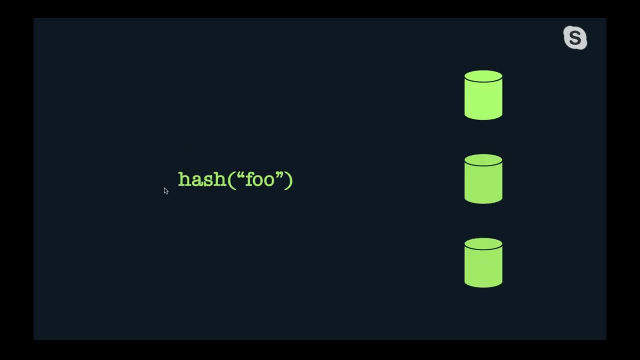 So if I do a query like this- select star from C, where Cpartitionkey equals foo- What's going to happen behind the scenes is Cosmos is going to receive that query, It's going to hash that partition key and it's going to go find the individual machine that all that data lives on. 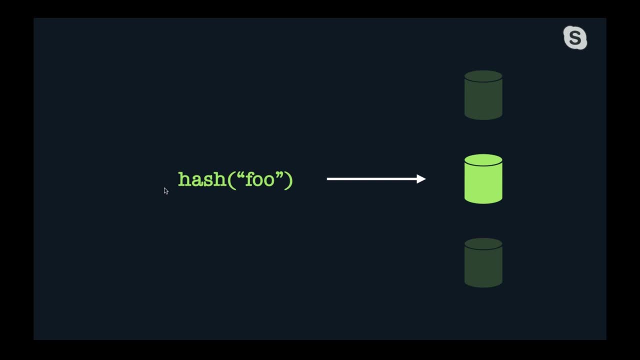 This is why partition keys and understanding them and where they fit into the system is very important, Because it means this is a very performant query. Every single time this query for any given partition key is executed, it's only going to run on one machine. 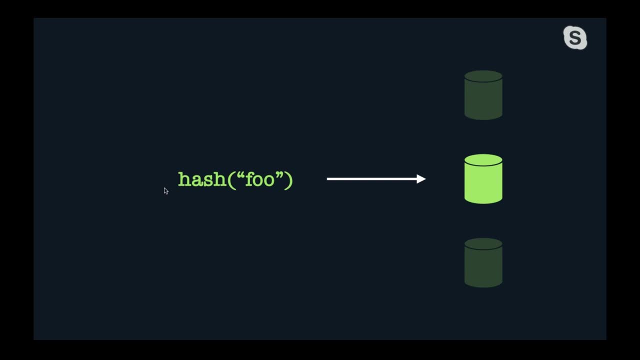 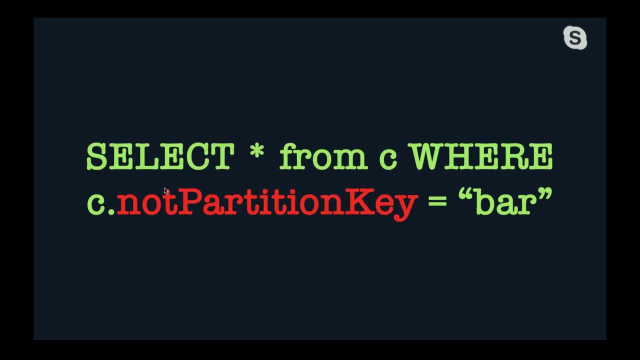 All of your data for that query is co-located. It's going to be very fast. It's not going to have any fancy processing to do either on the back end or on the SDK side. But what happens if you do the reverse? 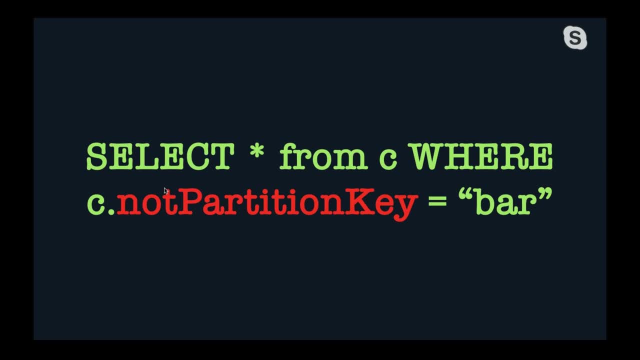 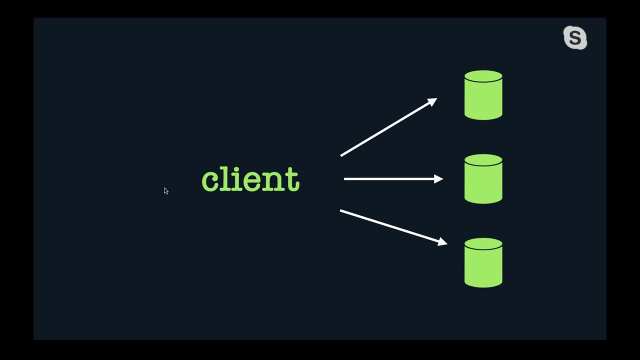 So we call this a cross-partition query. You query on something where you're filtering by something that is not a partition key, And what happens is is the client then kind of takes over And it ends up finding a list of all your partitions from the back end. 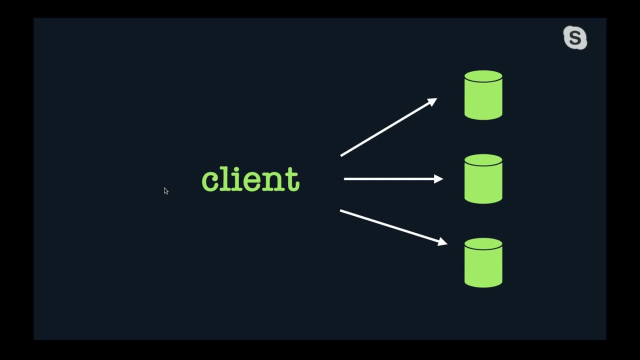 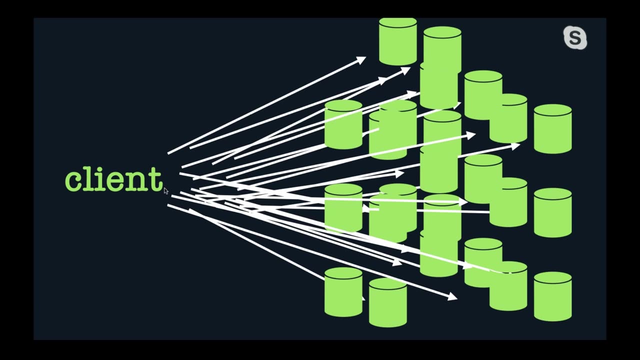 And then it goes and executes them against each physical partition. Now Cosmos is unique in that it sort of provides this for you, But what happens is, over time, as your data set grows, you end up doing something like this: You are having a cross-partition query in your application. 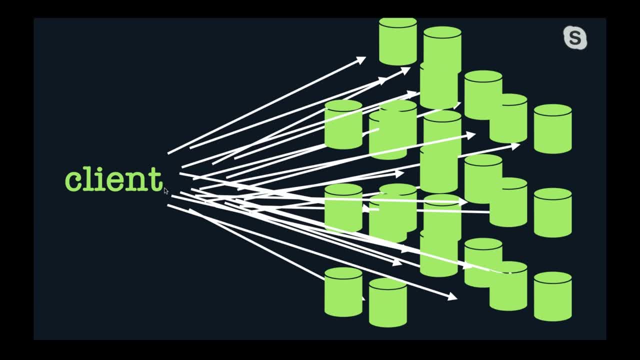 And you go from 1,000 users to 100,000 users And suddenly that query will slow way down because it's having to execute way more queries, Individual queries against individual partitions, Even if some of those partitions don't contain any of your data. 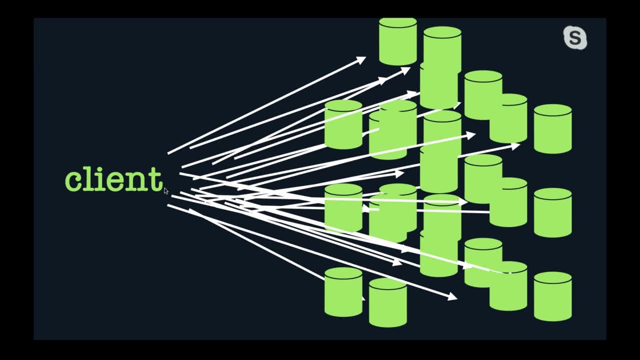 Also. this can cause problems on the client because it's executing all of these requests in parallel And there's ways to tune this a little bit with the various SDKs. But we often see people running into client issues as well because they're having to process. 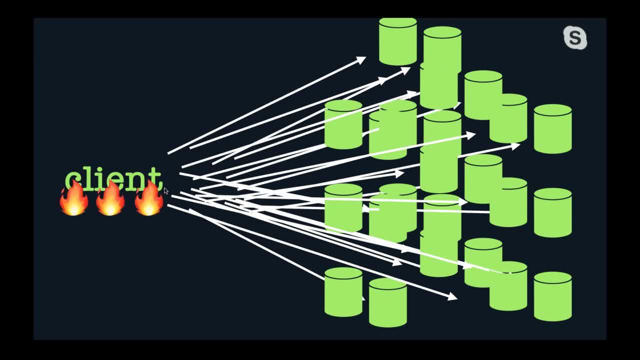 all these results and burning up CPU cycles and doing all kinds of stuff like that. So cross-partition queries something to be avoided. So what happens if you do a cross-partition query? Well, if you do a cross-partition query, 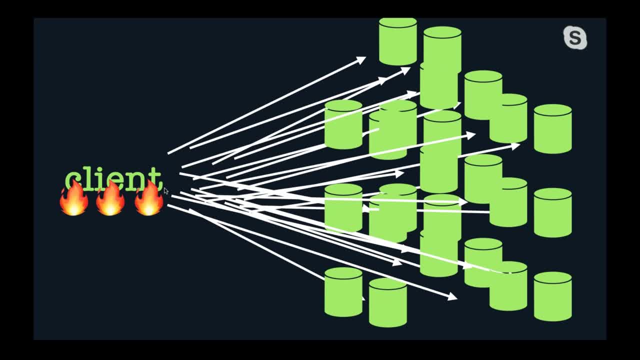 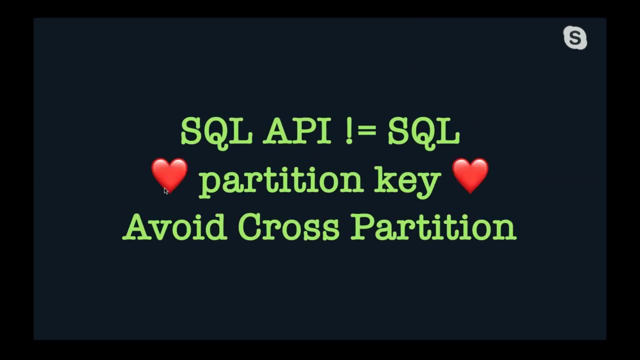 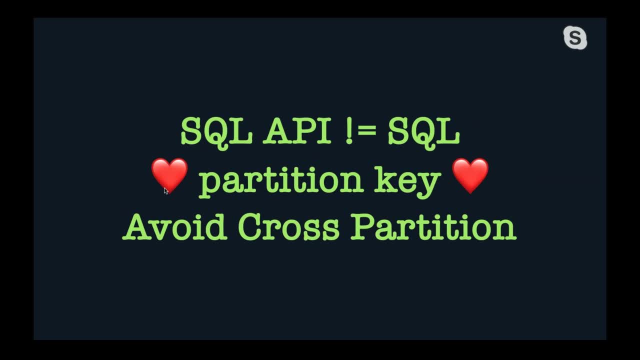 into the relational modeling part of this. But SQL API does not necessarily mean that it's SQL. The partition key is very important to understand and you're going to learn to love it as we get through this presentation, And we want to avoid cross-partition queries. 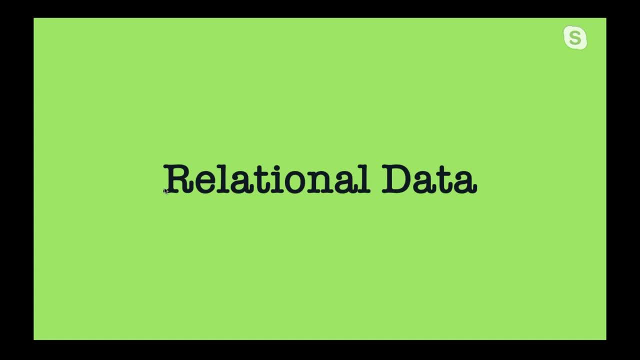 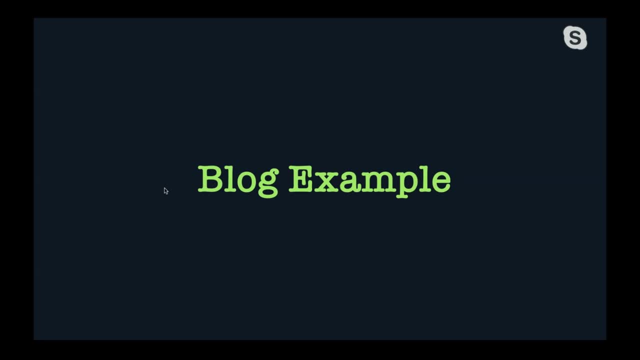 So that kind of gets to the meat of what I'm going to talk about today, which is the relational data modeling. I'm going to use a simple example of a blog, So there's some key bits here that I don't want to lose. 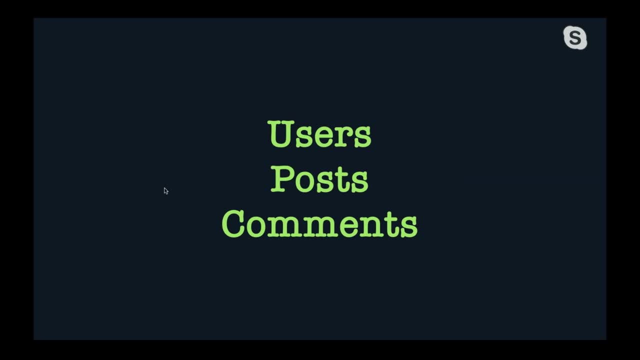 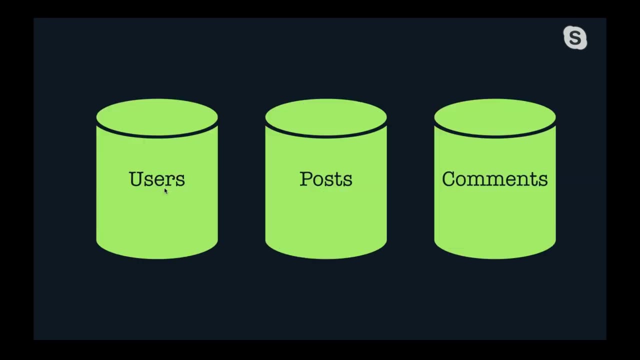 So I'm going to try to keep the examples really simple. We're going to have users, They're going to have posts and posts are going to have comments. If you're coming from a SQL background, you might have a system already like this that has tables, and you might just hop over. 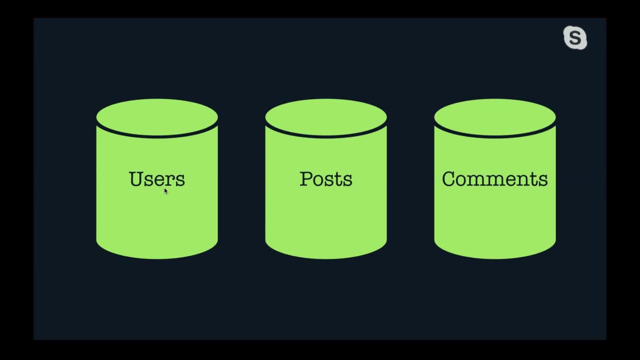 to Cosmos and create three different containers- a user's container, a post container, a comments container- And we need to provide partitioning information so Cosmos knows what to do. So maybe on users you'll partition ID, You can do this. 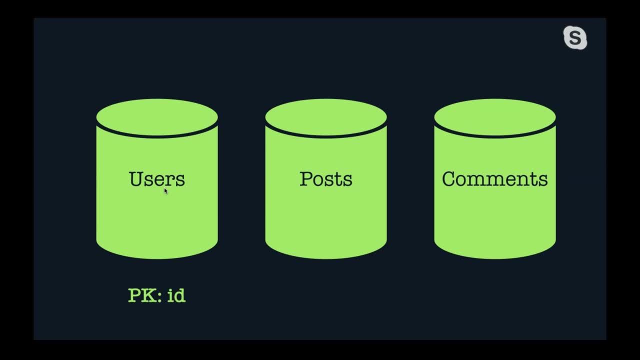 You can have your partition key and your ID need the same thing. It's actually, if it's possible for your system to work that way, highly recommend it. It'll be very performant because your data will be evenly spread across lots of partitions. 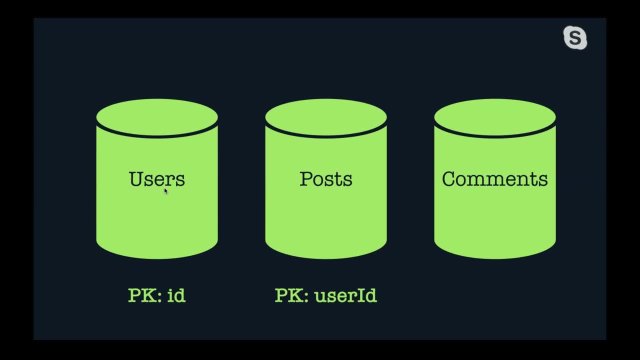 Maybe on posts. We want to make sure that we have a lot of data. Maybe on posts, We would partition on user ID in order to figure out, you know, like all the posts for an individual user. So we could provide that in order to just query an individual user's posts. 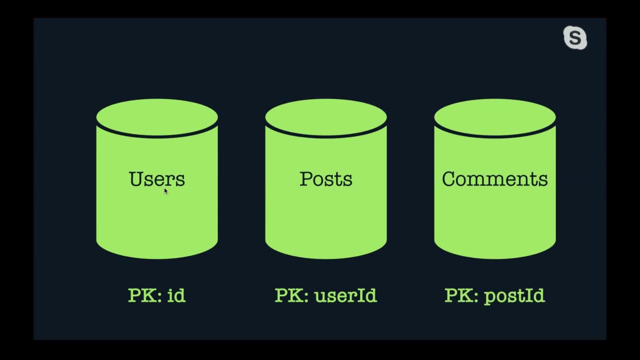 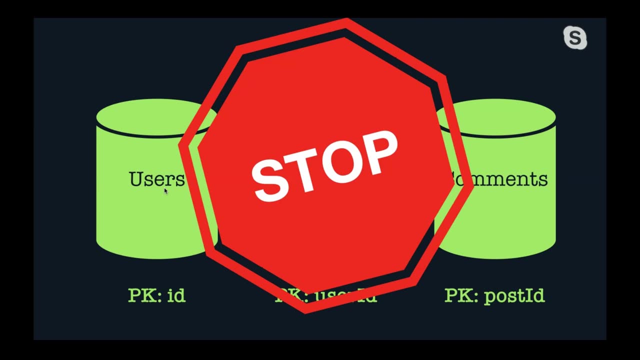 Similarly, a comments container could be partitioned on post ID so we can get all the comments for an individual post. You don't want to do this. I have misled you, probably over the last 15 seconds. This is not at all the approach that you want to take to modeling data in Cosmos. 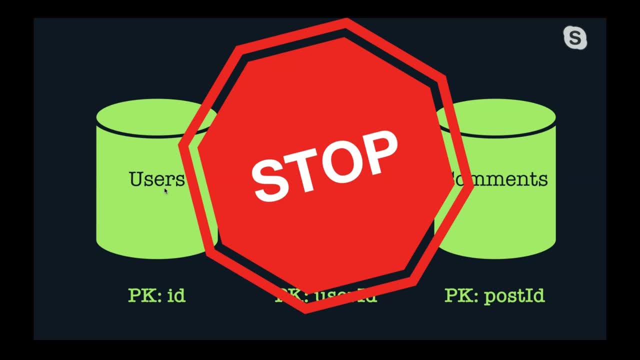 And it's tricky Because this is sort of the reverse of how you're taught to model data, especially coming from a SQL background. I mean, it's how I was taught to model data when I was doing a lot of Postgres work. 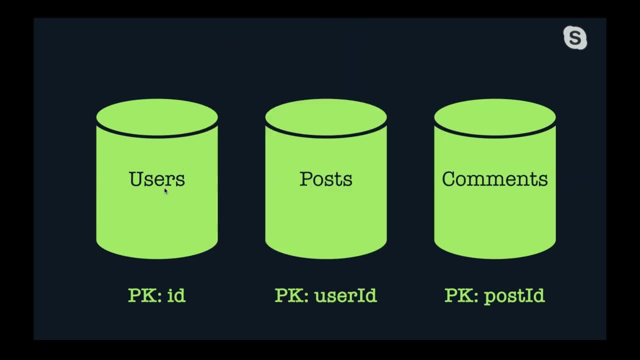 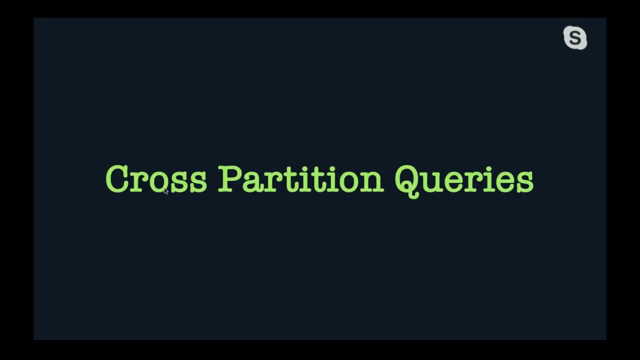 And it took me a while to understand that this is actually an anti-pattern, And I'm going to go into why. before I sort of talk about exactly how we should be doing things, There's a lot of cross partition queries that will crop up here. 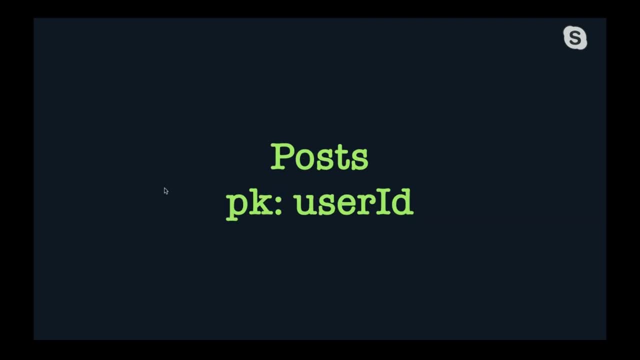 Right. That's why this is going to be a problem. Let's look at one example: Our posts. They are partitioned on user ID. Imagine if we want to find one Right, One post. Well, how do we do that? 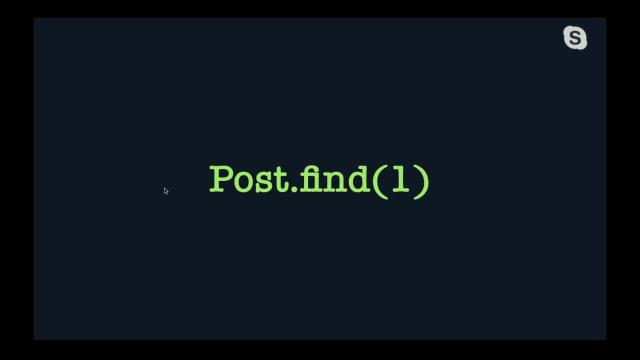 We only have the post ID. We don't have the user ID. We don't have enough information to uniquely identify that post. It's still possible with Cosmos to make this query, But the problem is it's going to result in a cross partition query. 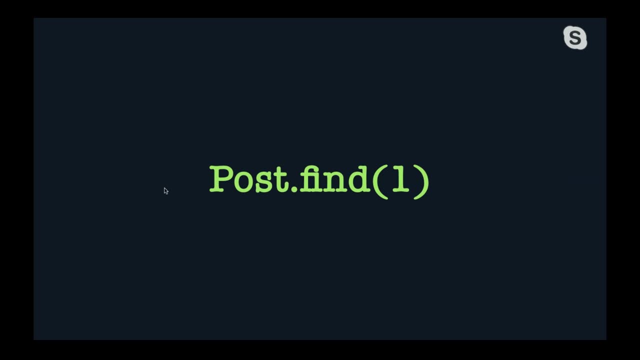 If you have hundreds of thousands of posts that are stored across several machines, it's going to talk to every one of those machines in order to find an individual post, And you can imagine that that would be very slow as well as problematic if you have users. 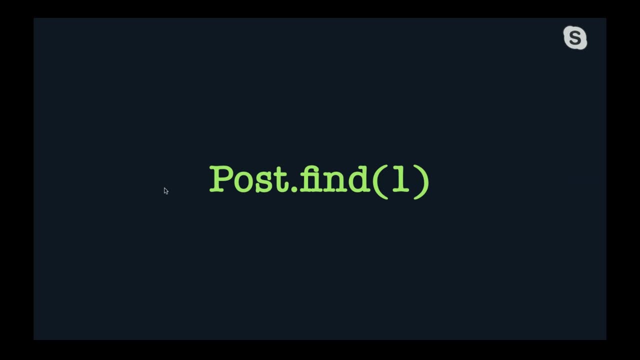 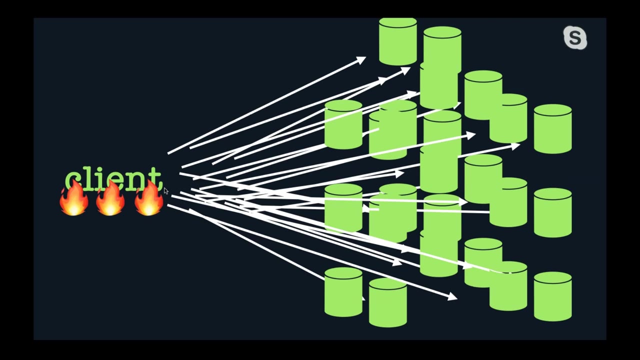 who are coming to your blog and they come right to a post page and they don't have user information and you don't have user information and you just need to find a post by ID. This is the kind of situation we'll run to. As your wildly successful blog becomes successful, you will have this problem. 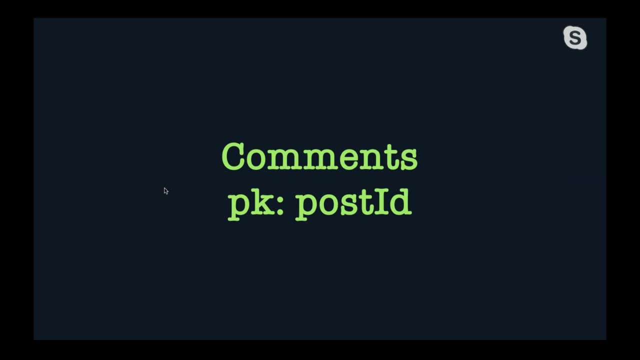 Comments. Another example of where we're going to run it at cross partition queries. We decided originally to partition it on post ID. It seemed to make a lot of sense at the time. We still can't find an individual comment. It has the same problem as posts. 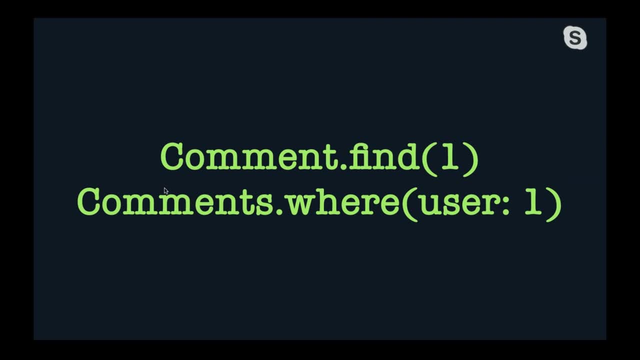 But what if we want to find all the comments that belong to a user? We might want to give them the ability to see that on a page, or edit a list of comments, or see a list of comments. even These are all going to be problematic. 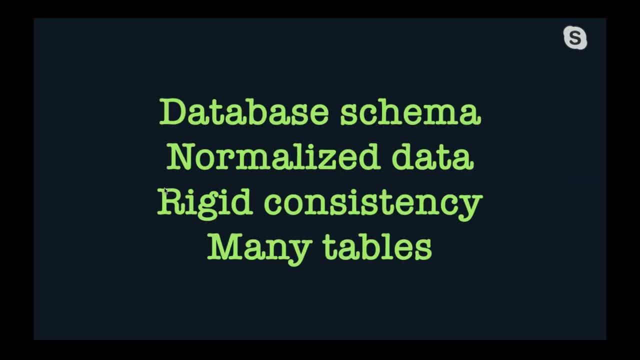 And it's because we sort of brought this SQL style thinking, which I kind of like. There's a lot of things that go into SQL style data modeling, But in my opinion these are kind of the critical bits to understand. In SQL we rely on databases to drive the schema or to store the schema. 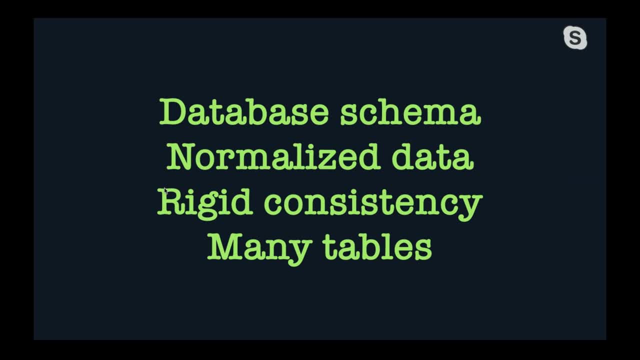 We normalize our data, so we want to keep only one copy of it when at all possible. We have usually pretty rigid consistency with SQL. We have very strong guarantees, We have transactions, things like that, And as a result of normalizing our data, we also have many different tables. 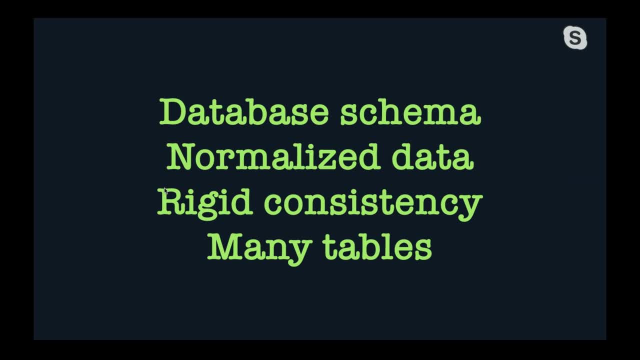 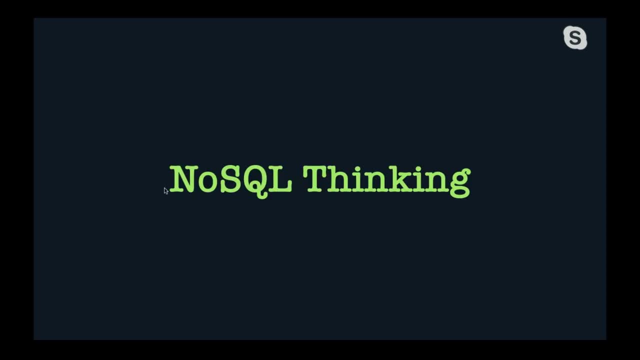 And that's sort of what led us down this path of doing lots of cross partition queries, No SQL thinking Right. So this is now the new approach we're going to take And this is what I'm going to do. This is what I'm going to talk about the rest of the time. 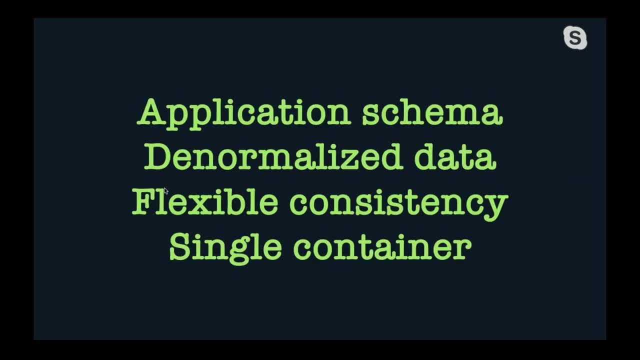 We need to sort of flip what we were taught to do on our heads. First off, the application is going to drive the schema right. Cosmos doesn't have a schema. It's not going to enforce relationships. We're relying on an application to enforce those kinds of things. 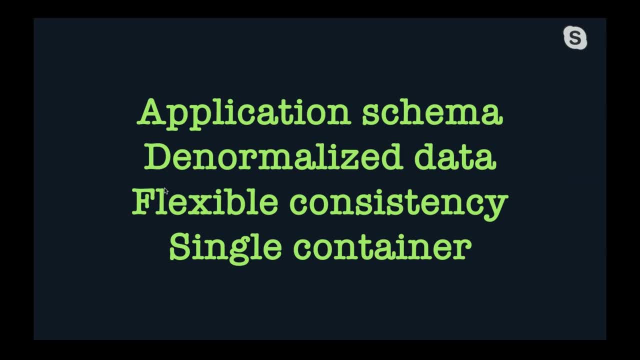 We're going to de-normalize data, So we're going to take data and potentially store it multiple times, And then we're going to have flexible consistency. So one thing that I definitely run into with users is that they say, well, I can't use. 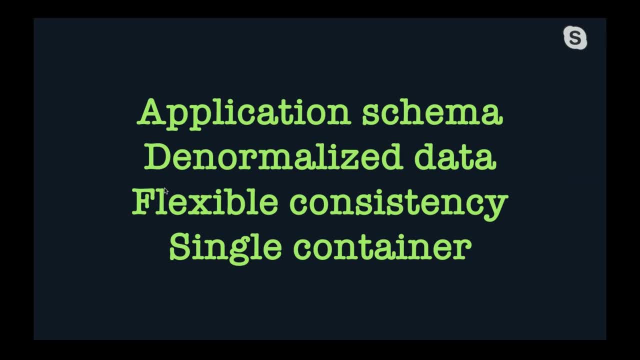 this, And so this isn't going to work, And it turns out that I think in practice transactions are not always necessary, right. If we write a couple documents and we need them both to succeed, we can just retry that right. That actually works for a lot of systems. 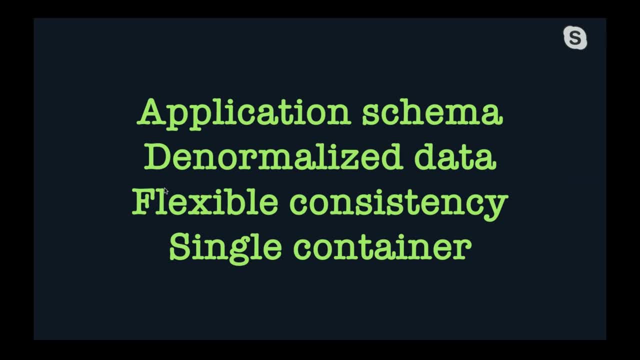 If you're maybe writing credit card transactions or something like that, you should look at doing something differently. But flexible consistency is an important term here. Cosmos does have the ability to do transactions, but let's go to a single partition, And so we're going to have flexible consistency. 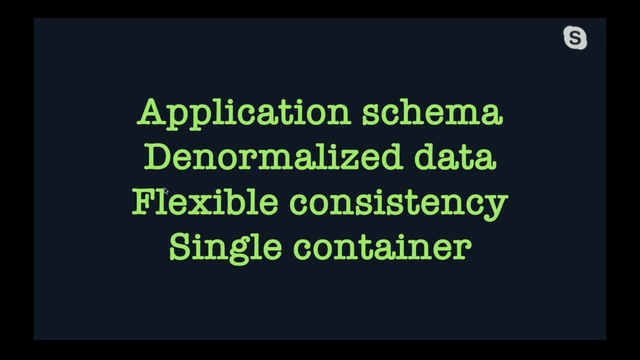 We're going to have the ability to do transactions, But let's go to a single partition. Lastly, we're going to start with a single container. We're going to put every single piece of data into one single container. It's going to look like this: 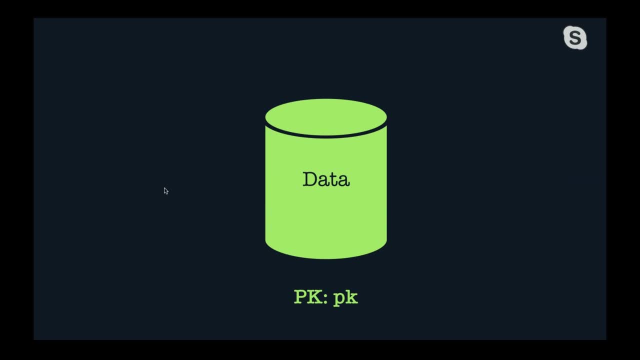 And I'm going to sort of explain how this is going to work here in a minute. But our data is just all going to live in our data container And our partition key is just going to be partition key. I've sort of taken it and shrunk it down to just PK everywhere to help stuff fit on slides. 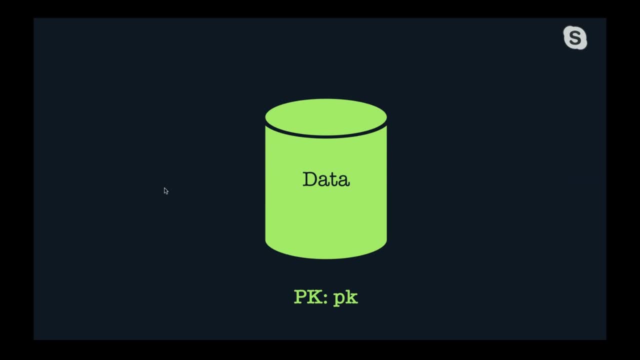 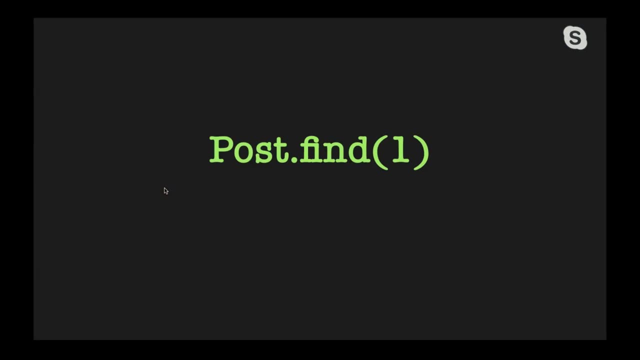 But you can really use whatever you want to call it here, like underscore, partition, key PK is fine too. It really doesn't matter, And Cosmos will let you set whatever you would like. So let's go back in time now and revisit some of our things and how we're going to model. 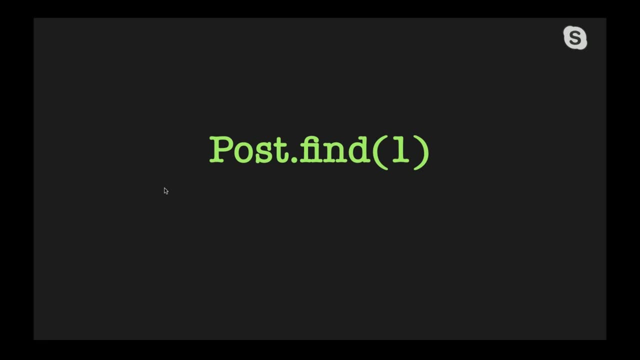 them in Cosmos. So finding an individual post. This was problematic before as it was causing cross-partition query, And what we're going to do is, when we create a post, we're going to do what we did for users: We're going to store the ID and the partition key as the same value. 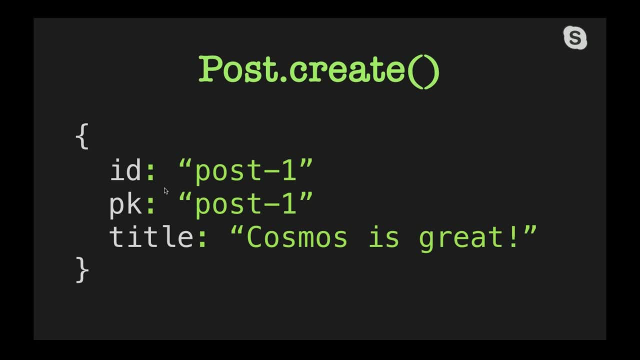 Right, Right, And we're going to do really efficient, fast point reads on any of our top-level objects. We're going to do the same thing for comments: Right, Post comments and users all now will have this document that stores kind of the primary. 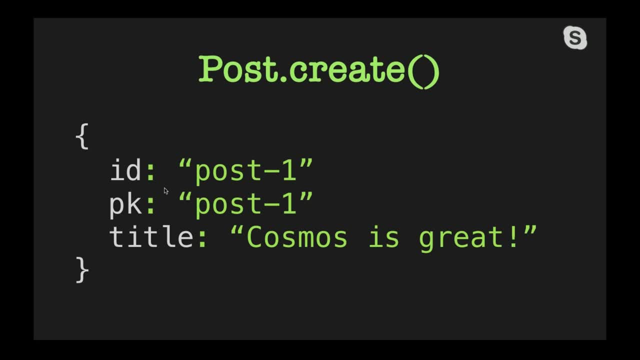 document for the top-level entity And it's going to store all of the information we need and we're going to be able to get it fast because we can uniquely identify it in the system. We know both ID and partition key because they're the same thing. 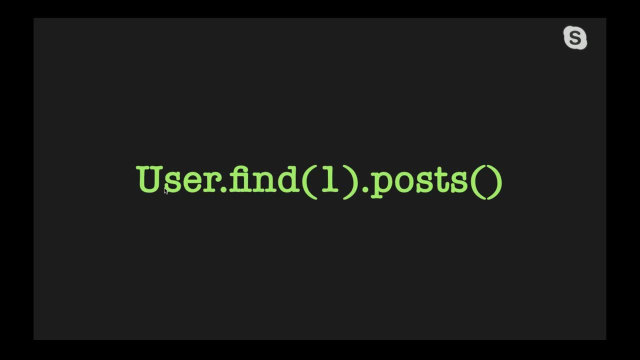 It's going to be fast. Now let's get into the relationships between these documents. If I have a user and I want to find all their posts, that's a good starting point. What we're going to do here is we're actually going to store two documents. 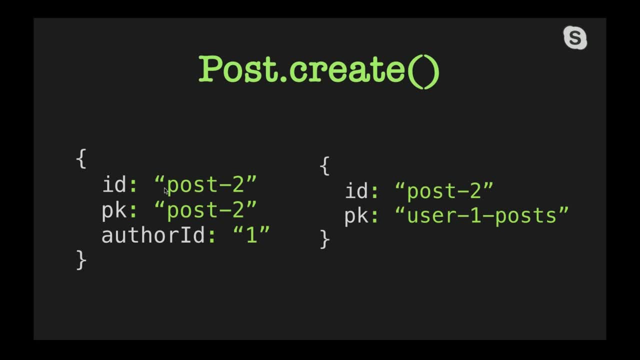 Right. So this is the first thing that we have to kind of wrap our heads around. is that when we create a post, we're actually going to create two different documents in Cosmos. The first is going to be the post itself, with all the post information, like the title and. 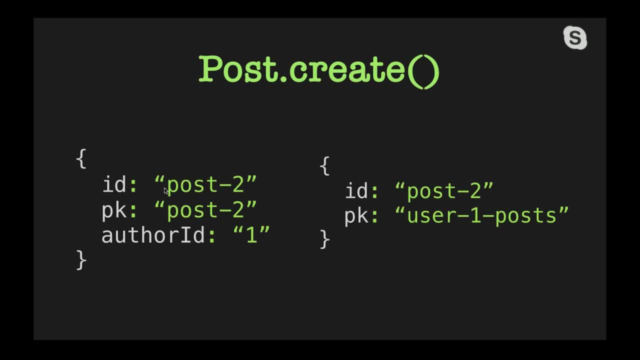 the publish that date and any other kind of post stuff. But then we're going to store a second document that links the post to the author. Ah, So the partition key here is going to be users-1-posts. You can see this matches up with the author ID on the other side. 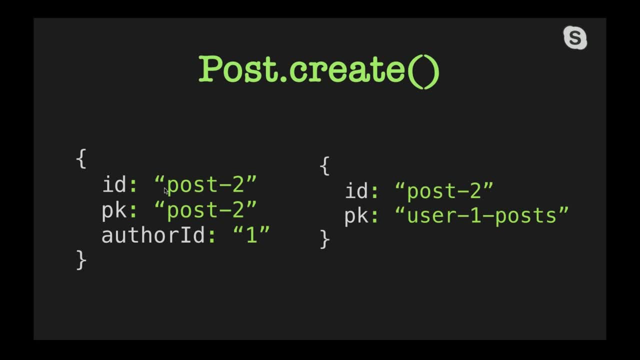 And then the ID. here is a pointer to the same ID as posts. So this document, because it's the same partition key, is going to serve as basically creating a collection of all the users' posts. So we're storing that information kind of in two places. 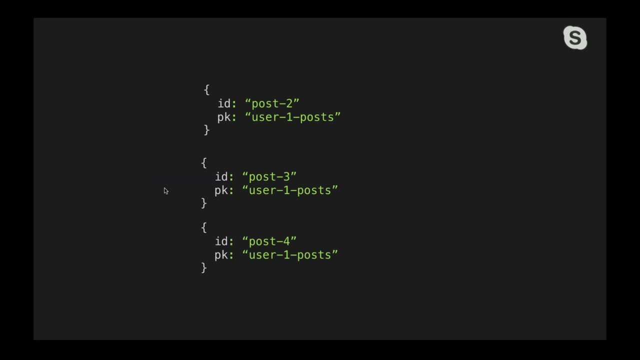 Right, We're not relying on the database to maintain that relationship, We're doing it at the application level. Ah, And if I created three posts, you can imagine that I would create three documents that look like this, All having the same partition key but then having different ID, pointing to the kind of 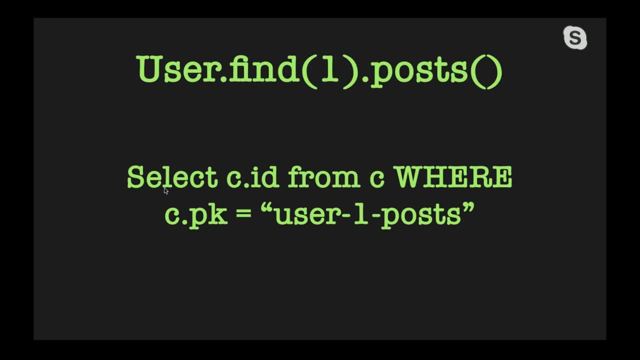 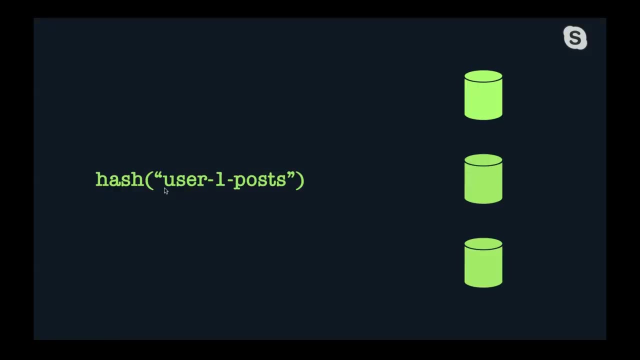 full post document. So now when I do this query, I'll do select cid from c, where partition key equals user-1.posts. And the important thing to understand here is that this is providing the partition key information, So we know that. 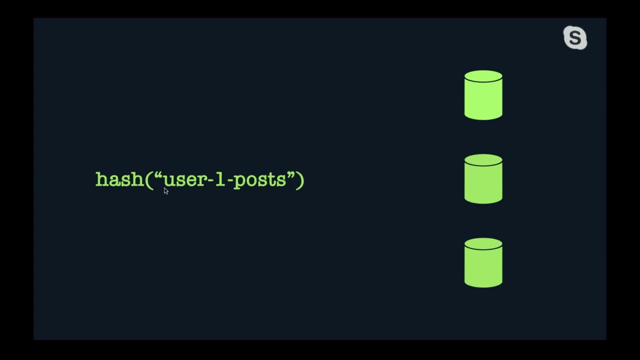 Ah, If we go back to our kind of previous example of how Cosmos is handling this, on the backend that query is going to execute against a single partition, right, We know it's not going to go across partition And this is sort of the beauty of this style relational modeling is that we might end up. 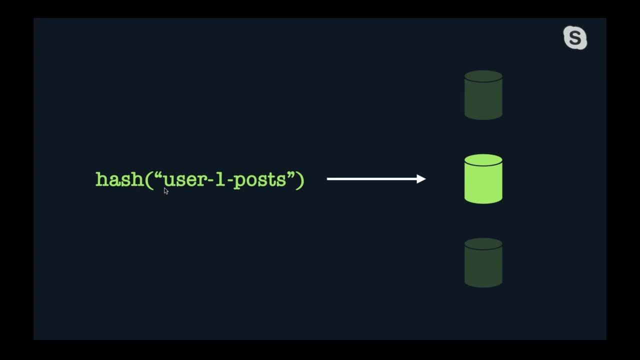 doing more queries because we don't have joins and things like that, But all of our queries are going to be very efficient and very fast because they're guaranteed to either be point reads or they're going to execute on a single machine. Ah, So this is what the return value would actually look like. 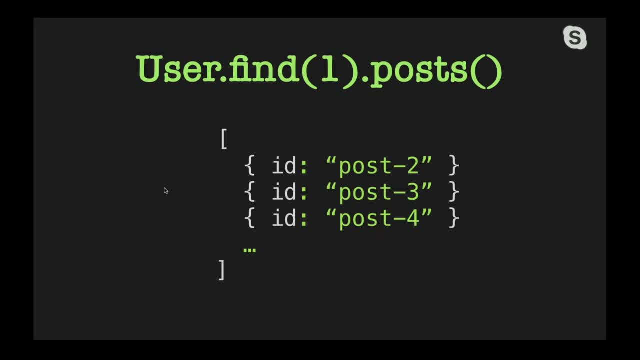 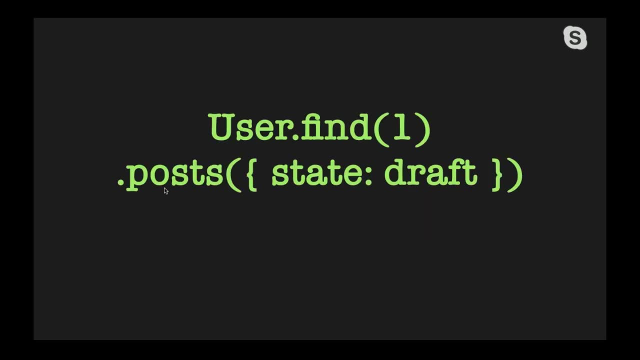 We get an array back of all the post IDs and then we might go fetch those posts individually and parallel in order to get more information from them. Let's expand a little bit more. So if I want to find a user's posts that are in the draft state, I'm going to do the same. 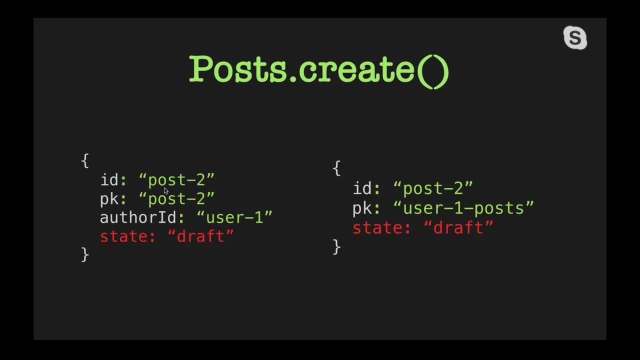 kind of thing. I'm going to create two different documents when I create a post And I'm going to again duplicate information. So before I'm sort of duplicating the relationship information. now I'm actually duplicating information that belongs to the post. 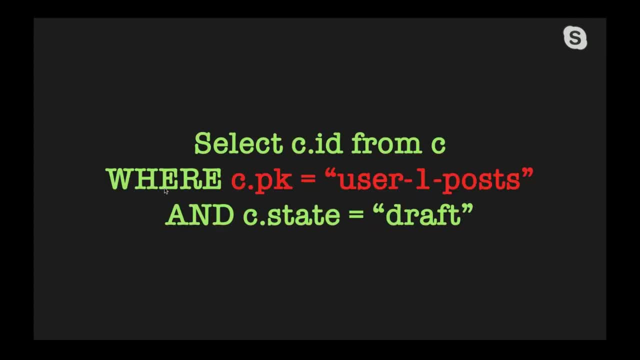 So this state I'm going to store in both places And what this allows me to do again is have a query that is scoped to an individual partition key and the state information I can also query on, because I know that that's going to execute. 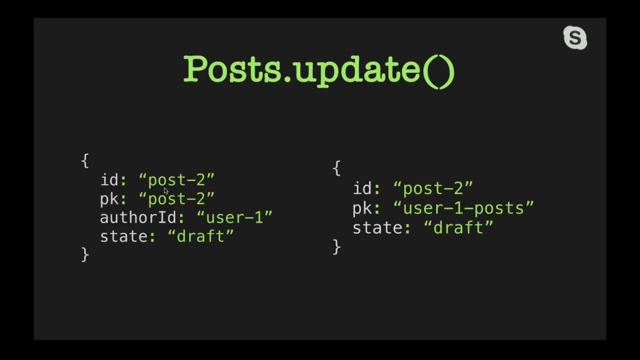 on one single backend partition. There's the gotcha, though, right? So if we do that, when we create the post, anytime we update the post, we also have to update both pieces of information. Ah, Both pieces of information in both places. 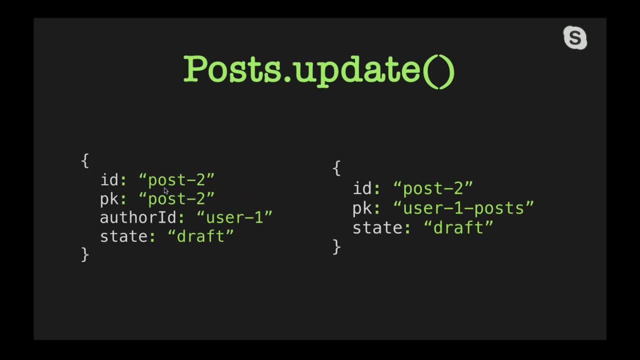 So this is sort of where it gets into, like the application becomes more responsible for maintaining the data consistency and the data integrity. right, You're trading speed for having forcing your application to do a little more work, And this isn't a bad or a good thing. this is just a trade-off, right? 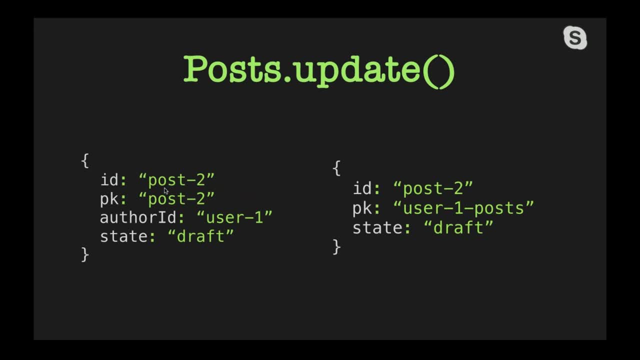 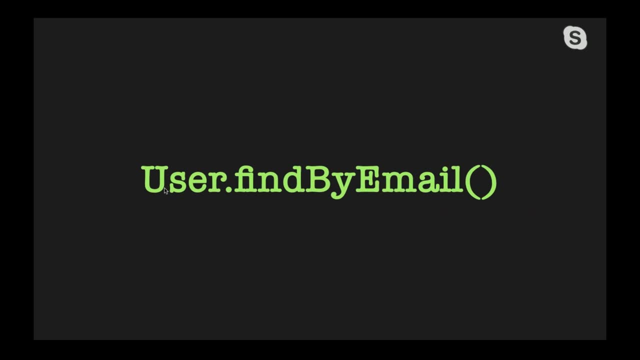 And it's understanding these trade-offs where you decide for your application what makes sense to do. Now, let's do something like A little more complicated than that. even So, what if we want to find a user by an individual email Right now? this would be a cross-partition query. 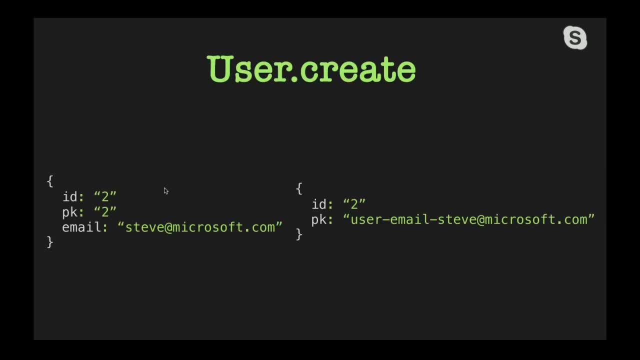 We would only. The only way we can uniquely identify a user is by ID. Again, we're going to store information twice. We're going to have two documents. The first one is going to be the actual user document with all the information. 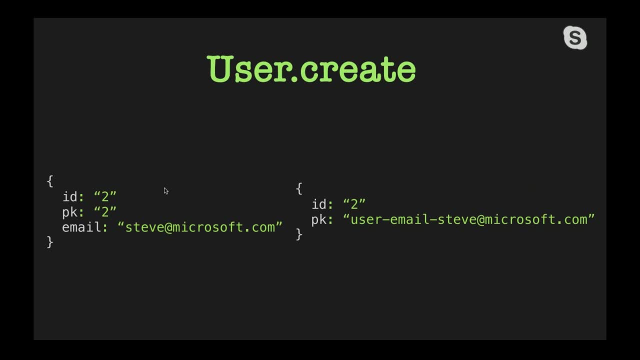 And the second one is going to be using the partition key, almost like a secondary index, right? So I would store my email in this, And then I would store my email in this, And then I would store my email in this. So what I'm going to do is I'm going to write that in there in a composite way so that 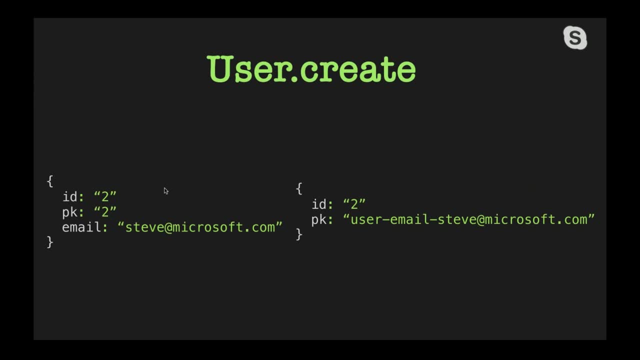 the partition key is user-email-myemail. This is actually not my email, just to be clear. There's some other Steve before me at Microsoft apparently, so I couldn't get it, But this is important to understand here, that this is allowing us to use partition. 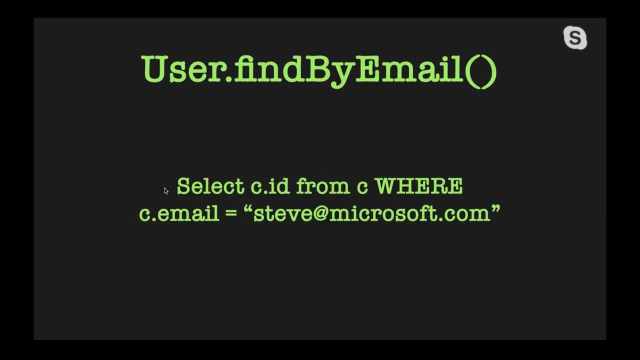 keys as secondary index on these attributes. So I can now, instead of doing this, which is a cross-partition query, right select ID from where cemail is, steve at Microsoft up. Now, if I do this query, I can actually do it as a single partition query and then I don't have 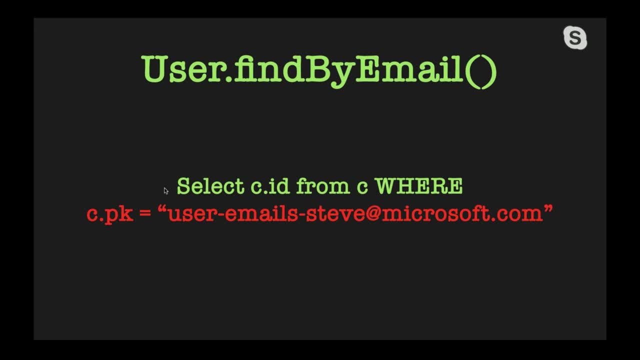 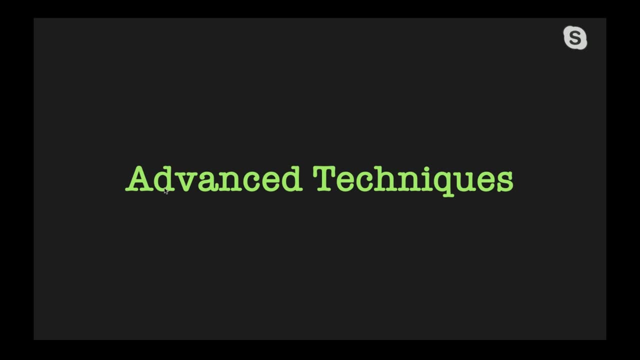 to worry about. you know, like that query taking a long time. There are definitely other things you can do. I've sort of just touched on the very basics today, but I think there's a lot to take away there, because it really sort of requires you to like reverse your thinking about how to store. 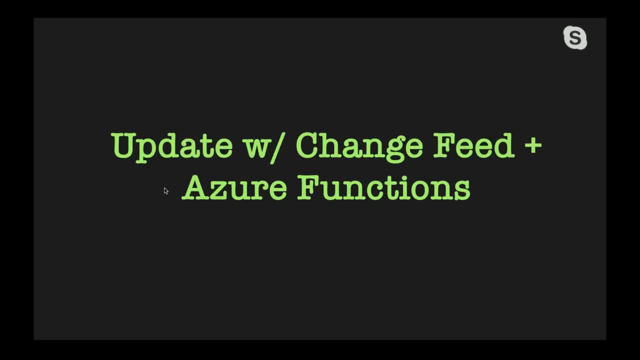 relationships and databases. But there are some more advanced techniques. Using ChangeFeed, as Santosh talked about earlier, is a really good example of how to kind of do more advanced things here. You can use Azure Functions plus the ChangeFeed in order to update documents later. 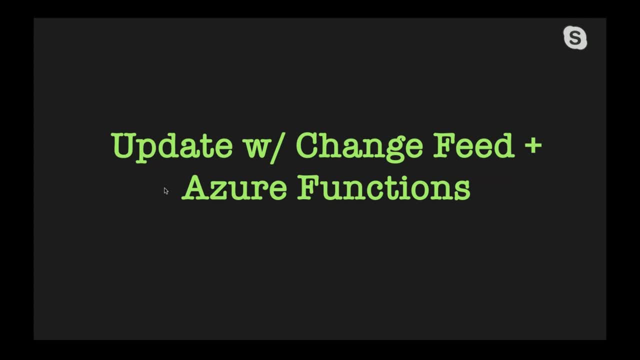 and sort of propagate out some of these changes to documents. You don't have to do them all right in your application or like all at the time you're writing the document. You might lazily update some information in other parts of their database, Materializecom. 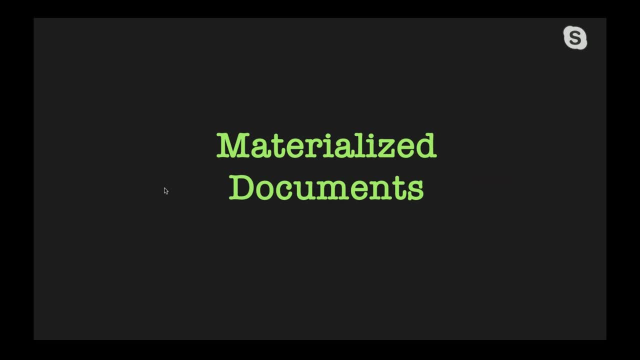 You can take documents and sort of materialize examples of them. The best example, I think, for a blog is if you wanted to have like a truncated version of the blog, maybe a little summary that showed up at the like beginning. We could potentially store this separately from the. 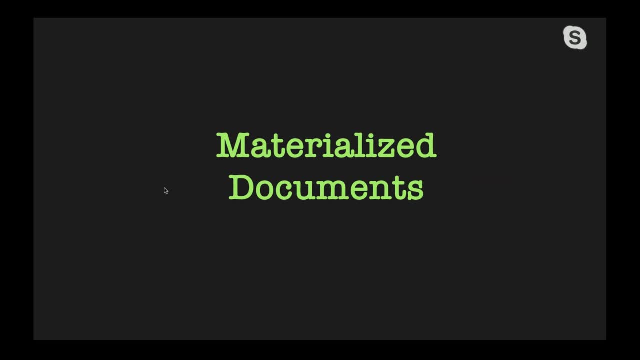 regular blog information and we would use Azure Functions to generate this truncated version of the blog every time somebody updates it. The last one is splitting up containers, So I talked a little bit about this at the beginning that you want to do a little bit more of. But if you want to, 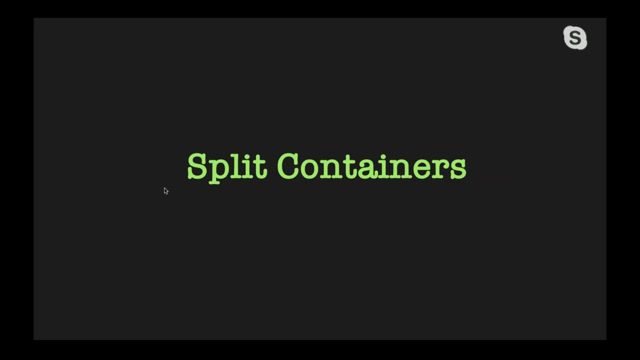 put everything in one container, but at some point it might make sense for you to split containers into multiple things, But I think I like trying to tell people to use this as an optimization. right, If you find some query is hitting one partition, even if it's not cross partition, but it's still. 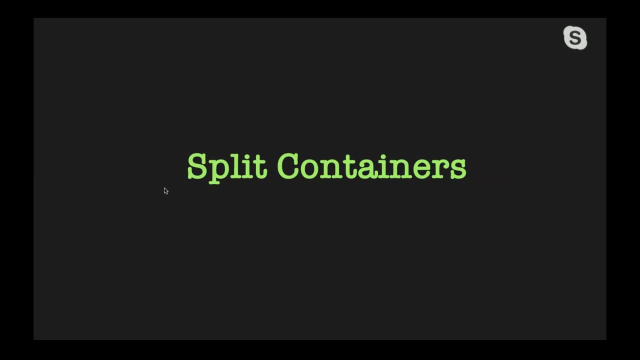 like heavily hit by your end users and you can't really cache it or something like that. you need to make that query work better. you can split that information out to a different container And there's no reason that you can't do that for any part of your data. But I think it's better. 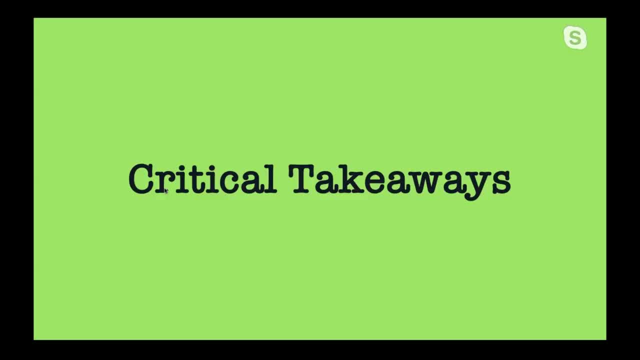 to start with one container and then sort of optimize over time. So critical takeaways: I'm just going to kind of recap a bunch of stuff that I've talked about and see what people have to say in the questions afterwards. But first off, start with a single container. I just realized I was 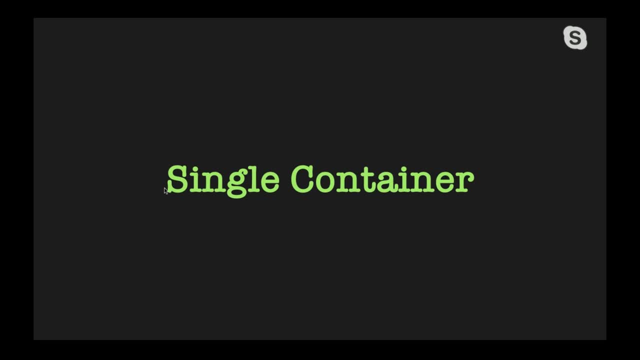 talking about splitting them, but start with a single container. I think that's the best choice for most people. What is the best partition key to use? Well, just use something called partition key, because you want to think about your partition key in a very flexible way. It is going to act as: 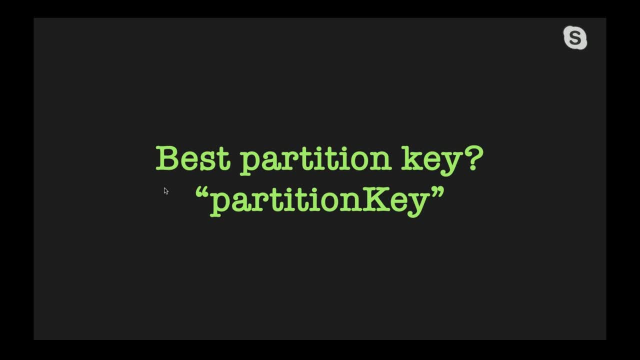 an identifier. It's going to act as an identifier. It's going to act as an identifier. It's going to act as an way to index things. It's going to act as a way to index things with, like, composite values. You can really do a lot when you just start stuffing data in your partition key Top level entities. 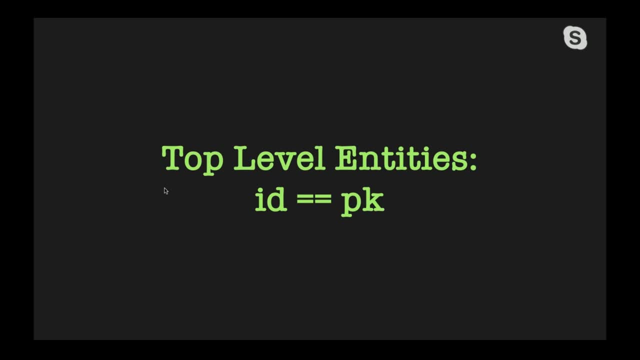 all of them, all of the top level models, should just have ID and partition key as the same thing, right? It's only when you're doing these secondary indexing operations or relationships that you're sort of having them be separate. Otherwise, this evenly spreads all of your data across all of your 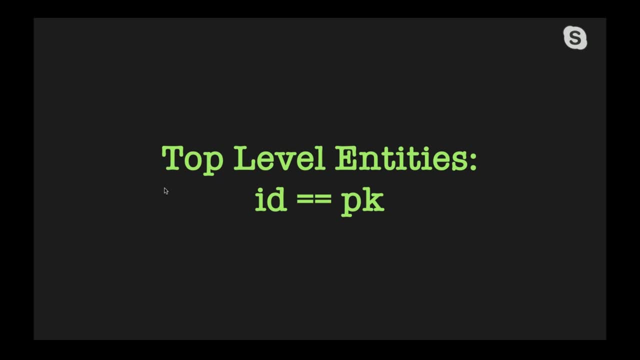 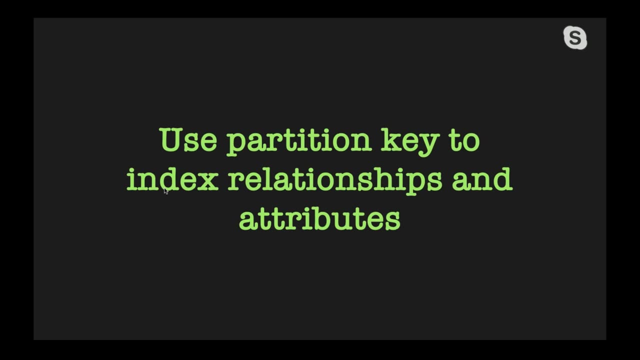 partitions, for just point reads, which is exactly what you want to do. You want to. you know you want to be able to do this. It's going to allow you to take advantage of the speed and sort of SLAs that Cosmos has. Use partition key to index your relationships and your attributes. 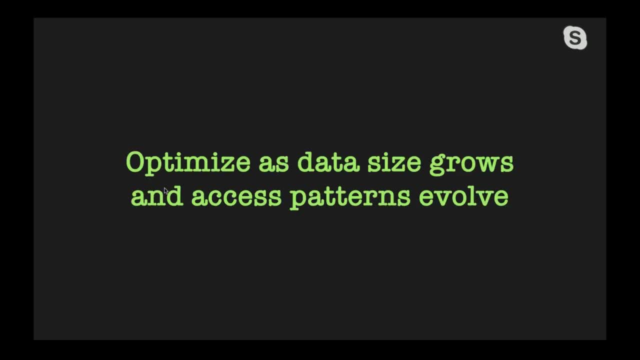 which I gave several examples of. And then, lastly, optimize as the data size grows. So I gave a lot of examples here of where you want to avoid cross partition queries, but that doesn't mean you couldn't start with a cross partition query and then later optimize it away. I think just to jump. 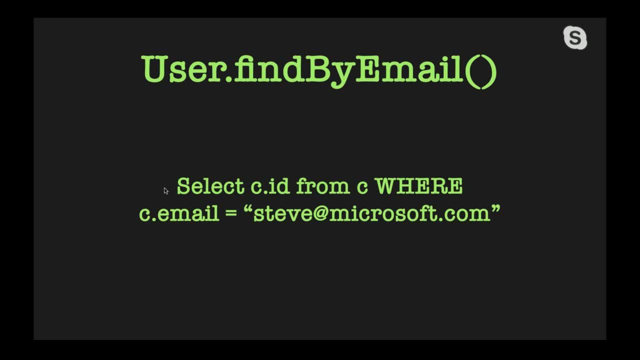 back a little bit. this is probably the best example Find by email. For a small number of users this might not be a problematic query at all. This is a cross partition query but if you only have a few partitions it might be slow or fast enough for a while. But when you start getting 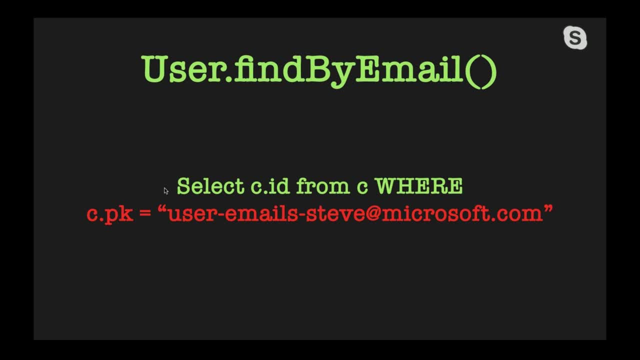 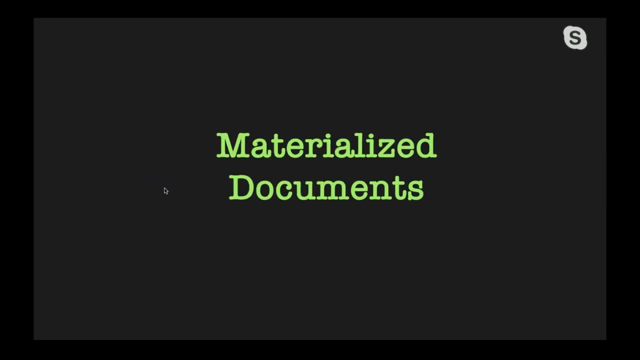 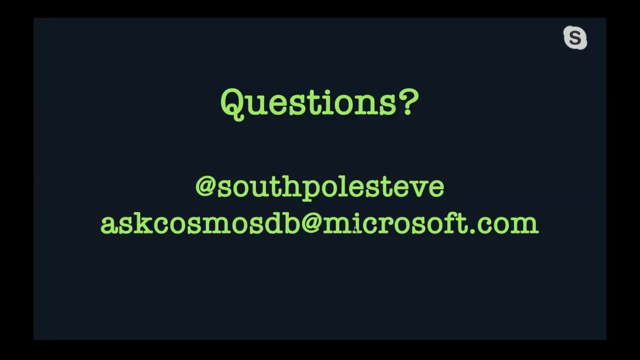 more users. you're going to want to optimize it into this kind of a query, which you can do. You can use things like change feed in order to replicate your data and sort of update these indexes later after the fact. Oops, I believe that's it actually. So that's at the end. 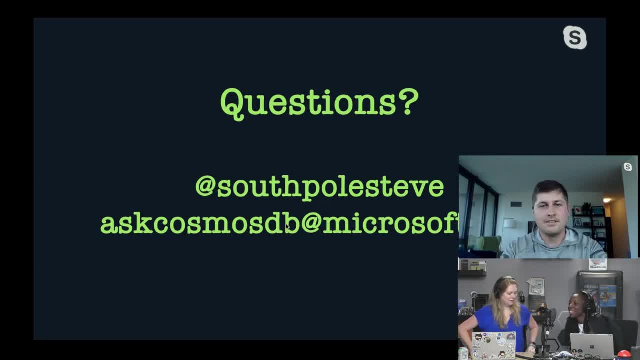 I'm happy to take questions from the comments. Thank you so much, Steve. So we have a couple of questions from people on the channel. The first one is: is there an upper limit recommended for the number of documents in a given partition? 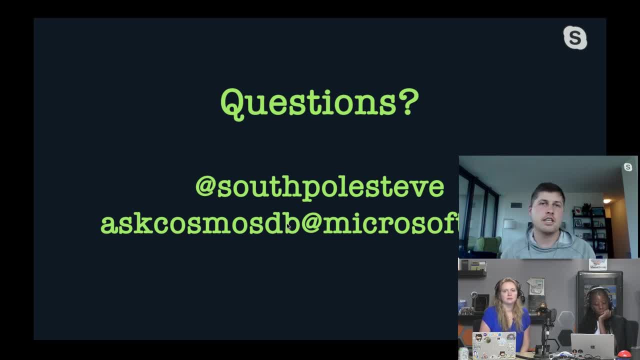 Yes, So in Cosmos one partition can hold 10 gigabytes, And one of the beauties of Cosmos is it will sort of handle that behind the scenes for you. It will split partitions in order to move documents between them and stuff like that, which is really cool. 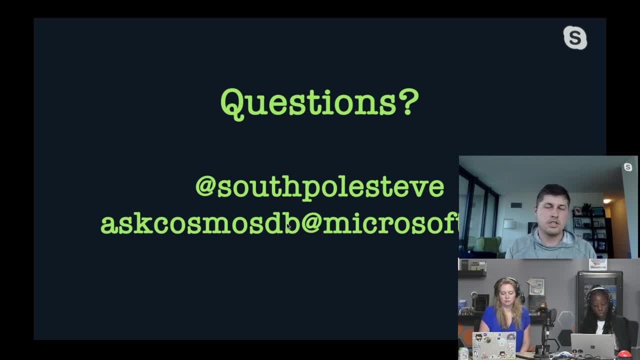 But you still can only hold a maximum of 10 gigabytes in a single partition. This can be problematic. There's different ways of handling it You can like. the best example I've come up with is like a chat application, Like most relationships in a chat application, you know. 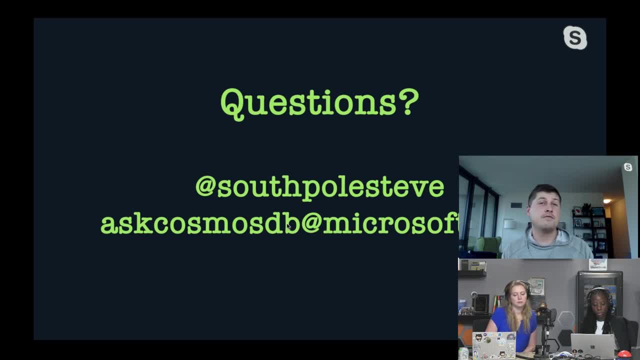 are going to fit under that 10 gigabyte limit, But if an individual channel has more than 10 gigabytes of documents, then you're going to have a problem. So more than 10 gigabytes of messages in one channel, And there's a lot of ways to handle that. So I'm going to go ahead and talk about that. 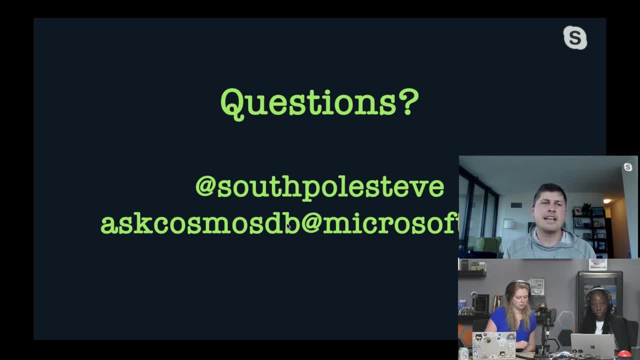 So I'm going to go ahead and talk about that. So I'm going to go ahead and talk about that, So I'm going to. there are definitely ways to do it. You end up sort of adding like a number to the end of the. 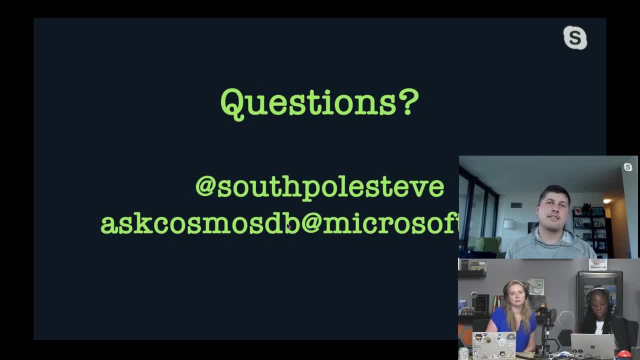 partition key name And then if somebody scrolls way back they end up going on to one of the old partitions. But you sort of like move your partitioning forward to accommodate that. There's some other strategies as well that probably go beyond this talk, But 10 gigabytes is kind of. 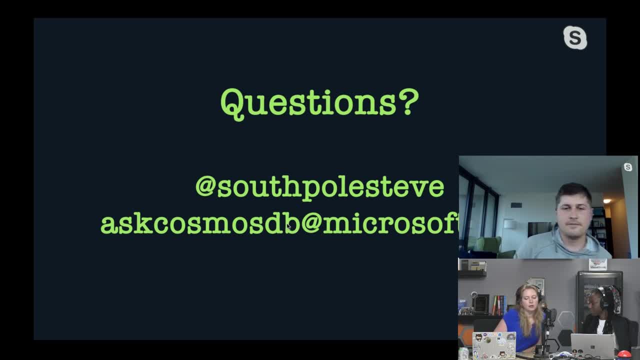 where this, you have to start doing fancier things. Another question we got is: why is this better than relational database? More scalable, Yeah, So I would say that that's probably the primary thing people are trying to get out of it.